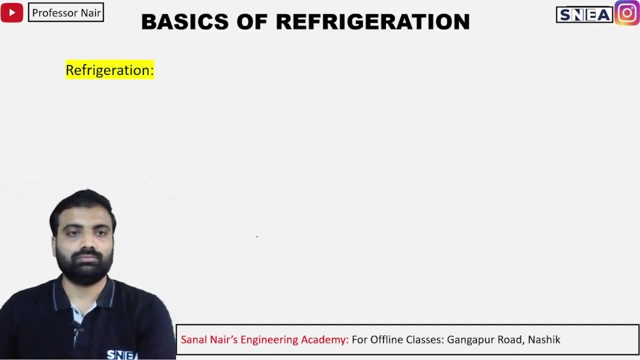 of Refrigeration. So, in order to understand what is the meaning of refrigeration, first of all we will learn about cooling. What is the meaning of cooling, students? Cooling means it is the reduction of the temperature, Correct If there is a hot body and if the temperature of that hot. 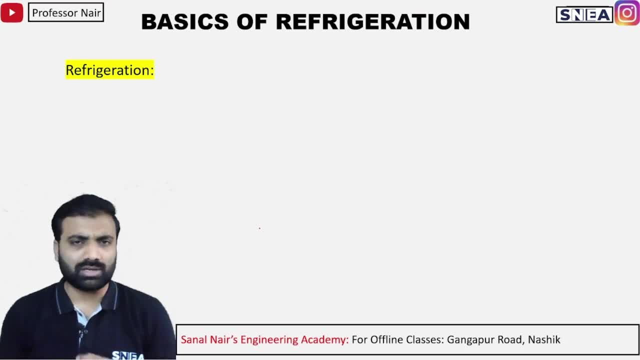 body has to be reduced, then we will call it cooling. So what is the difference between cooling and refrigeration? In refrigeration we can maintain the temperature. What do we call temperature? Preventive temperature? So we will show you temperature. 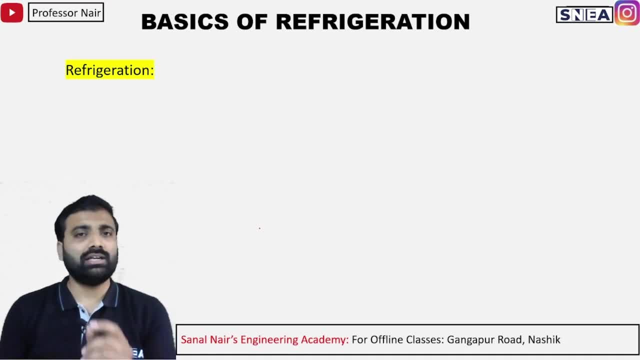 What can we do? We can maintain the temperature at a desired temperature. For example, if I put the temperature of AC at 24 degree Celsius, so it will set at that temperature only. So actually refrigeration is a cooling. Refrigeration has cooling, but at a desired temperature. 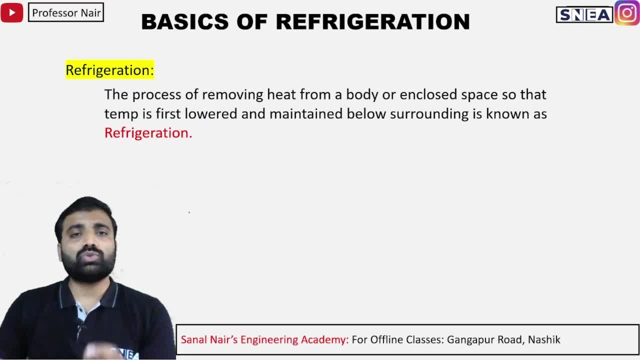 So the process of removing the heat. we are going to remove the heat from a body or an enclosed space, So there will be a body. For example, if I will draw here a body, what I have to get out of this body is heat. 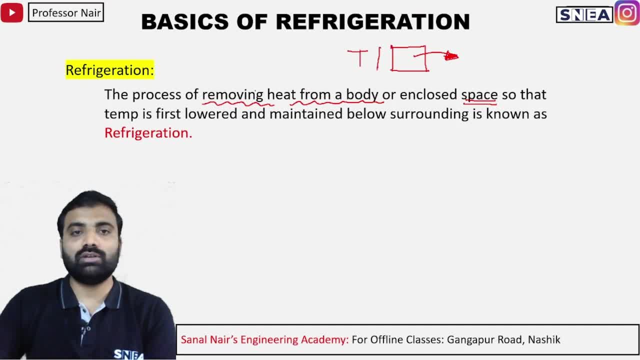 If I will remove the heat, its temperature will get lowered. So it is cooling, But remember it is a cooling Refrigeration is going on. So the temperature is first lowered- And this is important, students- And maintained below surrounding The temperature which is going to be there. they are going to maintain below the surrounding temperature. 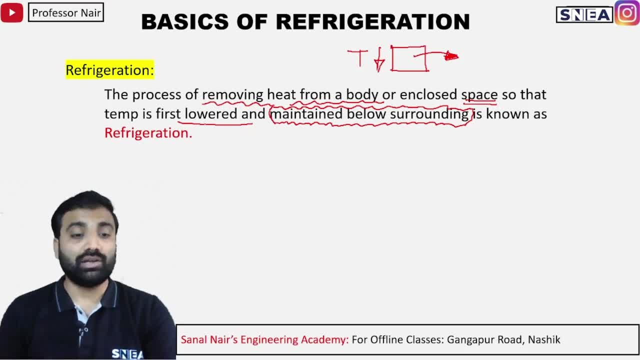 So that is called as what students? that is called as the refrigeration process. I hope that you are understanding the refrigeration First of all, understand that what we are going to study. So in this video series, First of all in this chapter, we are going to deal with cooling. 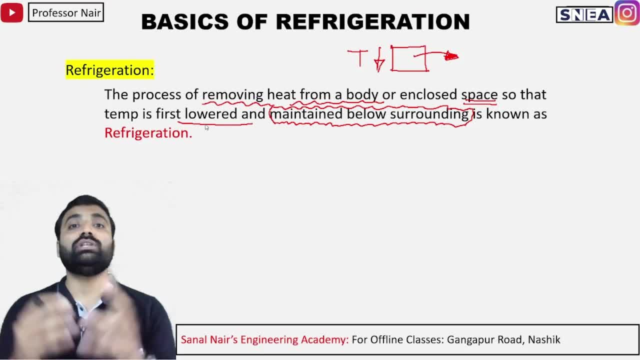 We are going to learn about the refrigerator, how the refrigerator works, and we are going to solve the numericals related to that also. So the body- the body here, students, the body from which we are removing the heat, that body will be called as what? 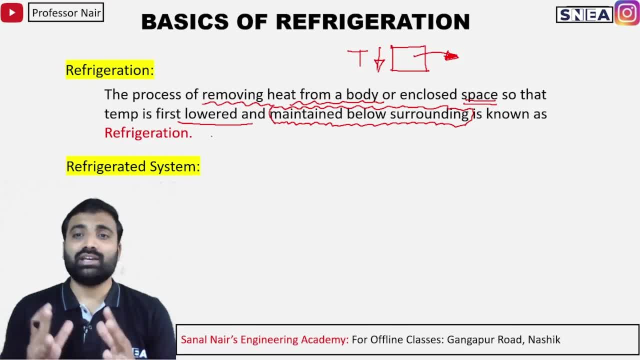 Refrigerated system. What do we call that body? Students, refrigerated system. We will say: are you getting my point? So the body or the system which we have to lower the temperature, then that system will be called as what? Students, that system will be called as refrigerated system. 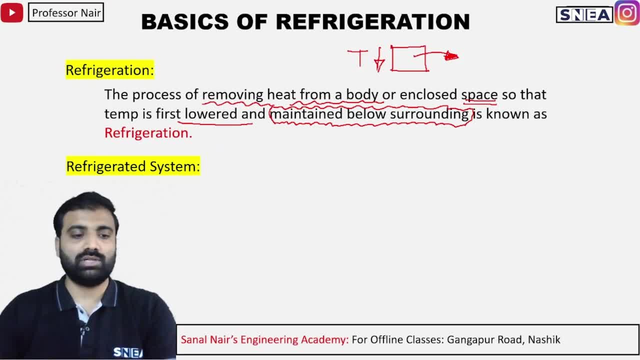 Let us see its definition. What will be its definition, Students? let us see The body will be called refrigerated system. The body or system which is maintained at a lower temperature, which is maintained at a lower temperature, is called as refrigerated system. 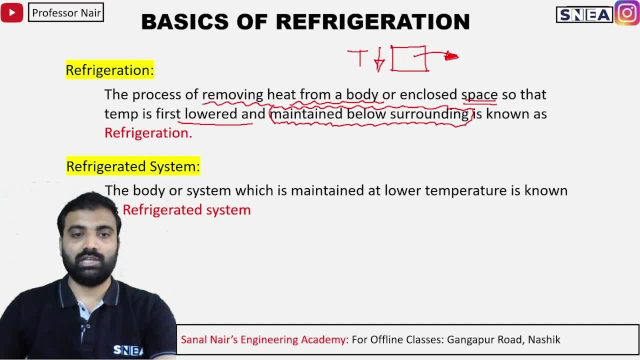 We will call it refrigerated system. Are you getting my point here? The body or system which is maintained, whatever the body is, whatever the system is which you have to lower the temperature, that will be called as refrigerated system. For example, if I am keeping an apple or if I am keeping an object inside, 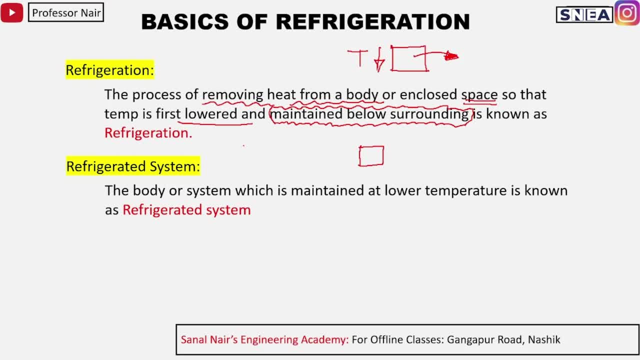 Refrigerator. So the apple or the body which is maintained, that will be termed as what, Students, that will be termed as the refrigerated system. Are you getting this point? The body or the system which we have to lower the temperature, that will be called as refrigerated system. 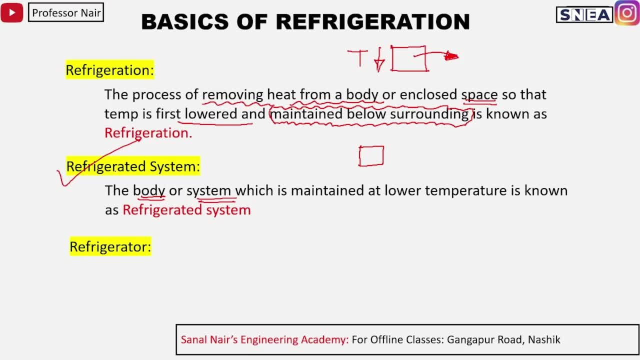 Dear students, let us see the next Perfect Refrigerator. Now, what is this refrigerator? The refrigerator which is maintained at home. that is your refrigerator. We know that. But what does a refrigerator mean? Refrigerator is an equipment, or refrigerator is a device where we can maintain the temperature. 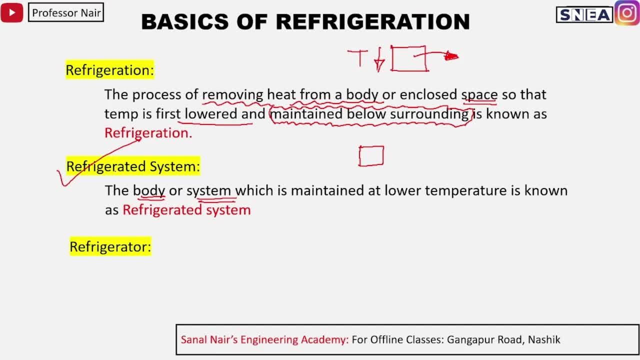 Refrigerator is a device in which we can maintain what, students, We can maintain the temperature. So let us see its definition. What is its definition? students? So let us see. The equipment used to maintain the required temperature is called as refrigerator. 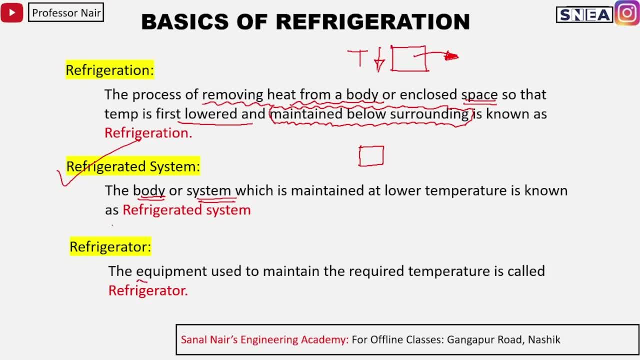 This equipment Or the device with which we can control the temperature. That device or equipment we will call as refrigerator. So are you understanding? Refrigeration is a process. Refrigeration is what students Remember. this Refrigeration is a process. 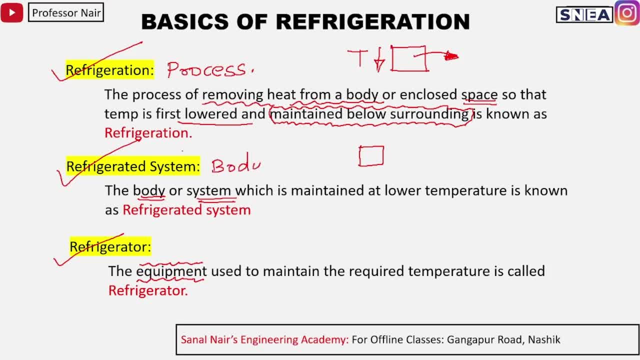 Refrigerated system deals with the body from which we have to remove the heat, And refrigerator is a device in which Refrigerator is a device in which Refrigerator is a device in which The refrigeration process occur. Refrigerator is a device in which the process of refrigeration is going to occur. 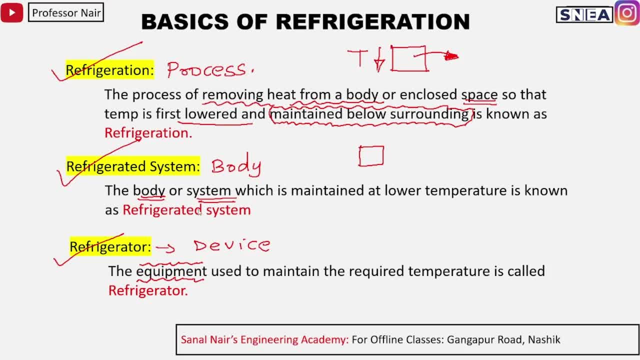 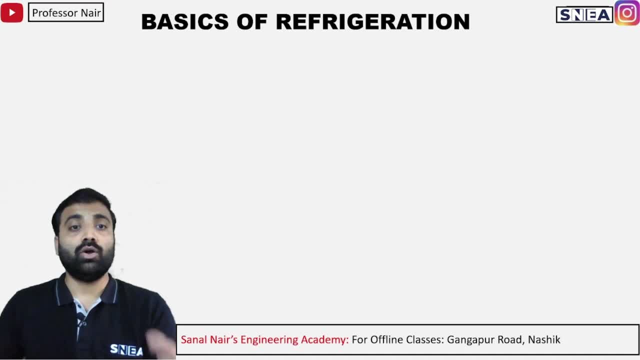 I hope that you are understanding this very well. So let us move on to the next part, That is, refrigeration students. So what will be the meaning of refrigeration? What will be the meaning of refrigeration That we had just studied here? 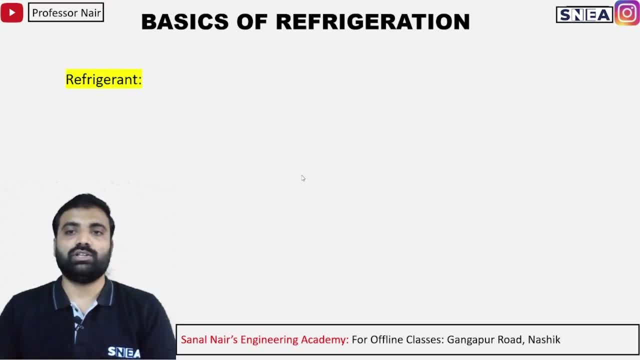 So let us move on to the next part: Refrigerant. So what is the refrigeration process? It occurs due to one substance. We will call that substance refrigerant, The working substance which is used, The working substance which is used To produce refrigeration process. 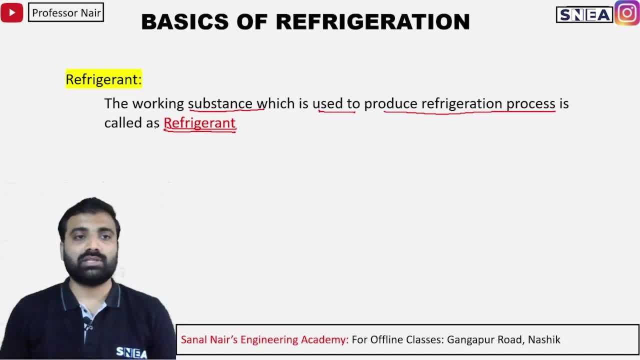 Is called as refrigerant, The substance due to which refrigeration is produced. We will call that substance refrigerant. Are you understanding? Perfect. Let us see the next part here: Refrigerating effect. The second part is refrigerating effect. Let us see the meaning of refrigerating effect. 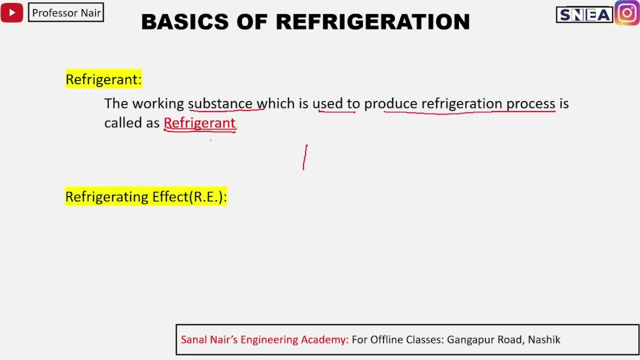 Consider this as a body. Consider this as a body. If I want to cool it. If I want to cool it, I have to remove the heat from it. I have to remove the heat from it, I will have to remove the heat. So the heat has to be absorbed. 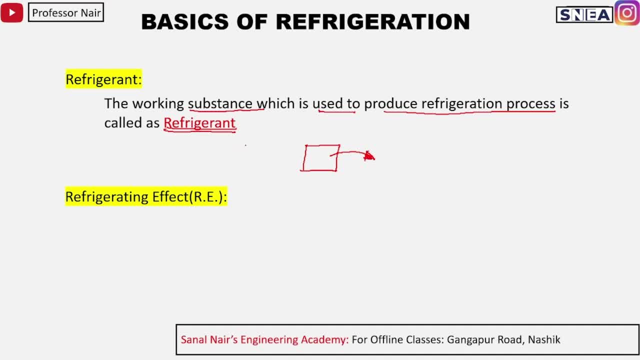 So the heat has to be absorbed. The rate at which heat is absorbed From a body or space, We will call that refrigerating effect. That will be called as refrigerating effect, For example. For example, I am removing here 50 kJ per second of heat. 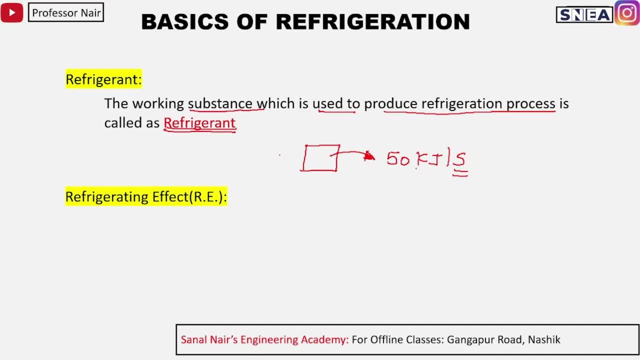 Means in 1 second. I will remove the heat. How much heat will I get? How much heat will I remove? I am going to remove 50 kJ heat, So that will be called as refrigerating effect. This is very important, For example. let us consider here A object. 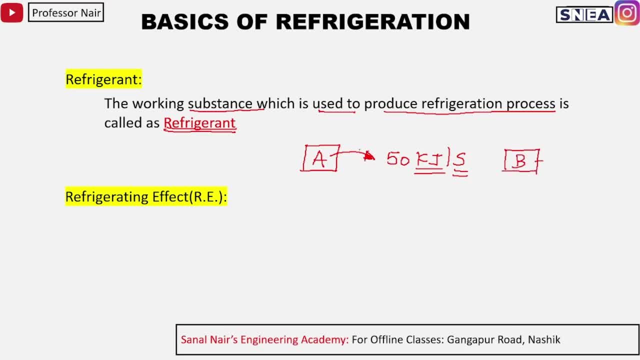 And this is your B object. Okay, Pay attention. If I am removing 100 kJ per second of heat from B object, What do you think? What do you think, students? Which object is going to cool? Which object will be cool? Will object A cool or B object cool? 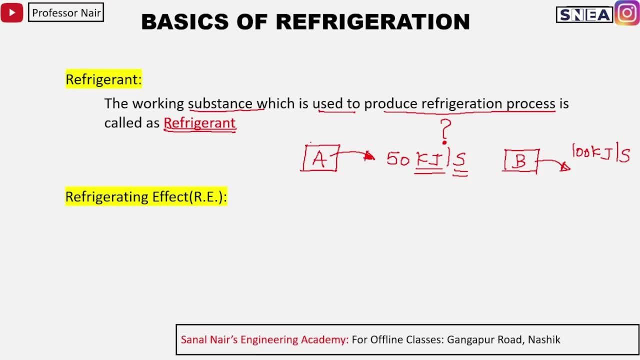 We are removing 50 KJ of heat from object A in 1 second And from object B we are removing 100 kJ per second. What do you think Which object is going to cool? So comment on the comment section. What do you think? 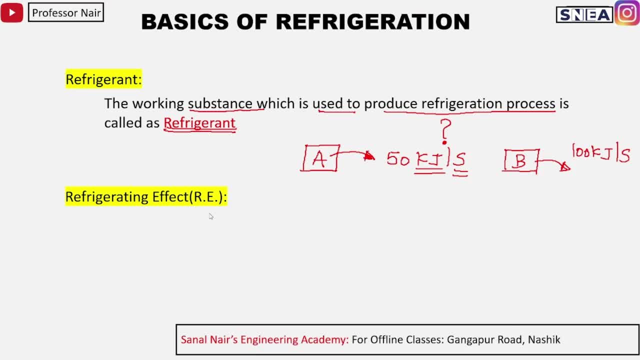 Please let me know. Everyone understood. So it is the rate of cooling we need. It is the rate at which heat is absorbed from the body or the space which is to be cooled. Us rate ko hum kya bole gaya. Us rate ko refrigerating effect kaha jata hai? 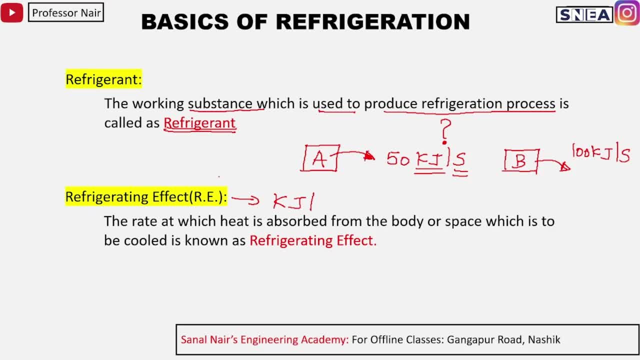 Thik hai. It's unit, students, it's unit is kilojoule per second, Kilojoule per second. So generally what happens is technically ek refrigerating effect. 1RE refrigerating effect equals to 3.517 kilojoule per second. 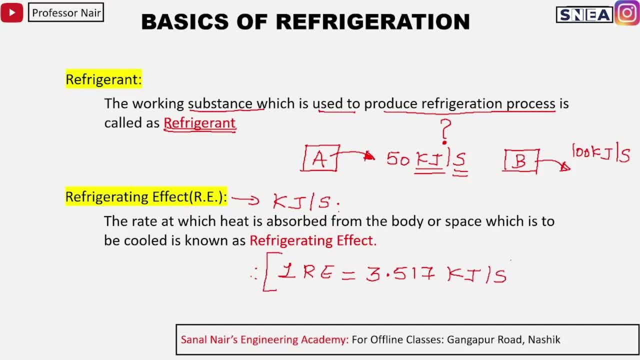 Yeh yaad rakho. Okay, this will be important students ki ek refrigerating effect ka meaning kya hai. It is nothing but 3.517 kilojoule per second. Generally it is also termed as a TR- tons of refrigeration bhi kaha jata hai. 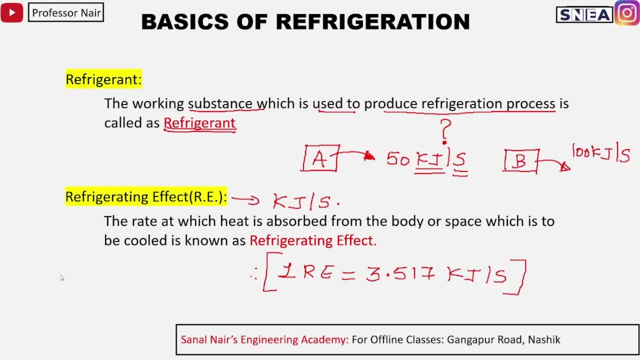 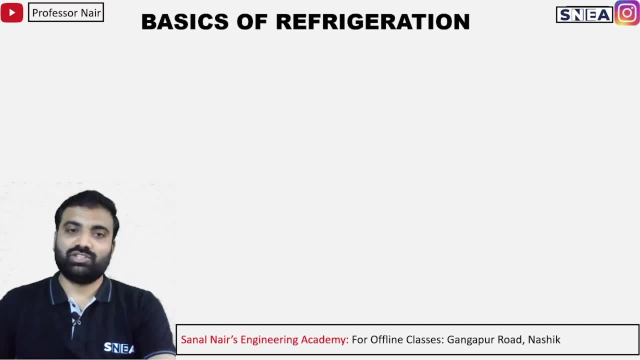 So what is that? tons of refrigeration That we will see in the next slide, students, Next slide mein hum Tons of refrigeration bhi dekhenge hai. So refrigeration, toh samajh mein aaya apko That. what is the meaning of refrigeration? 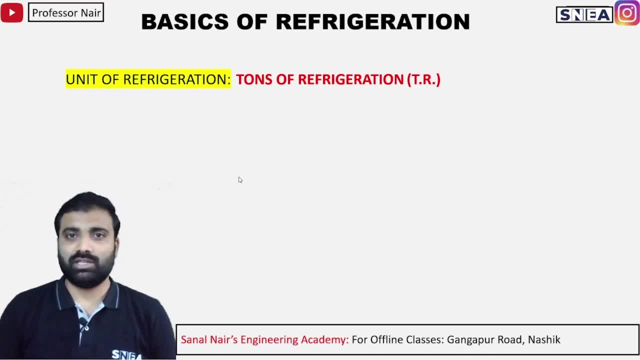 Refrigerated system. kya hai? Refrigerator ka meaning, kya hai? What is refrigerant And what is ultimately refrigerating effect? So refrigeration ka bhi unit rada Jaisa. power ka unit kilowatt. Correct mass ka unit kg. 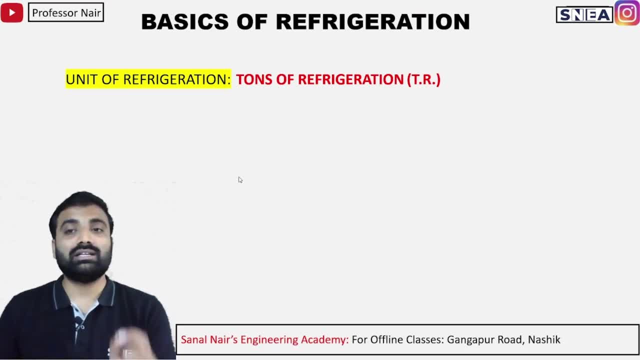 Similarly, refrigeration ka unit Reta hai students. Tons of refrigeration, that is TR Okay. so let us understand actually what tons of refrigeration means. Tons of refrigeration ka actual meaning kya hai? Let us understand in a proper manner. 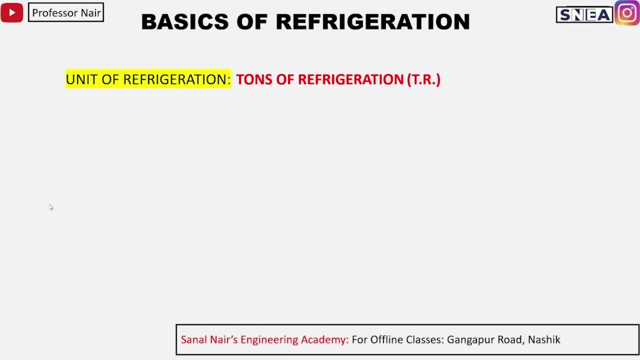 So, as you can see here, students, As you can see here, For example, I will consider here a water Water. consider karta hai That water is of one ton. Ek ton ka water hai Right, I have to convert it into ice. 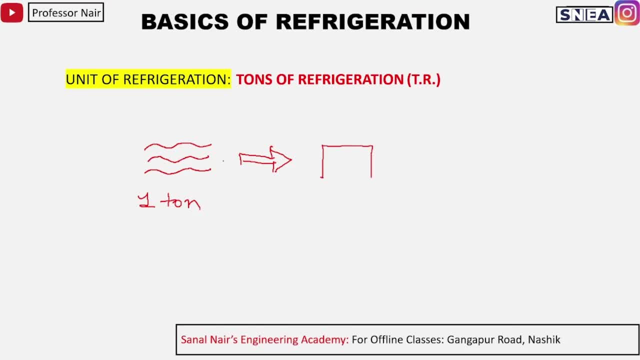 Okay, theek hai. So I have to convert that one ton of water into ice. So simple logic is that I have to remove here heat Heat kya karna padega students Heat? remove karna padega. I have to remove what. 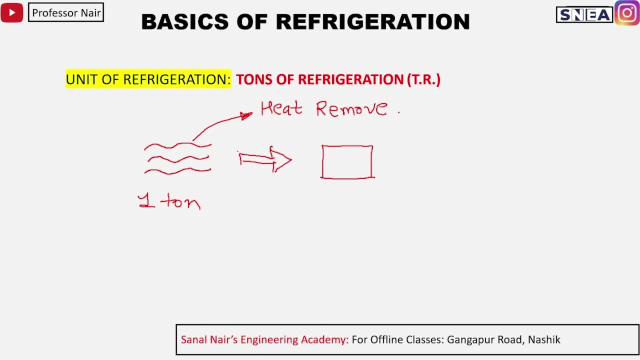 I have to remove the heat. When I will remove the heat? Yeh jo paani hai, yeh jo water hai. iska temperature kya hoga? iska temperature kam hoga When the liquid temperature reduces, students. when the liquid temperature reduces, it will get converted into ice. 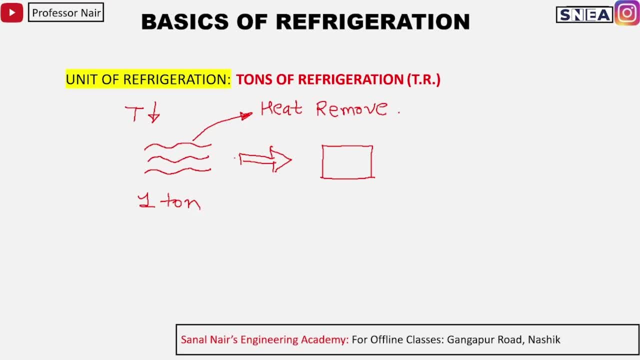 Chalo theek hai, koi baat nahi. But what you think? ek ton paani jo hai, wo turant convert hoga. ice mein, No, It will take some time. So time, kitta, consider koro bhai. 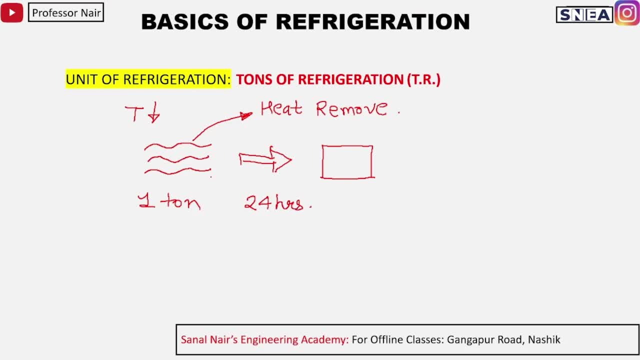 Time. consider koro 24 hours. So how many hours? I am going to consider 24 hours? Okay, But ice is forming. at how much degree Celsius? Zero degree Celsius, mein Matlab. zero degree Celsius, mein ice form. hone hi wala hai. 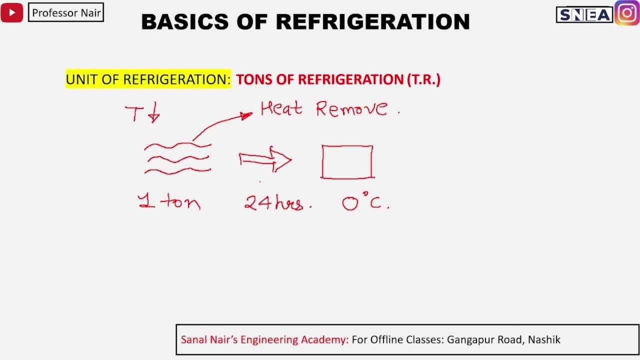 So what, in short, tons of refrigeration, is Ki aap kitna heat remove kar rahe ho. ek ton paani ko convert karne mein ice ke. What is the heat removed to convert One ton of water into ice at 24 hours in zero degree Celsius? 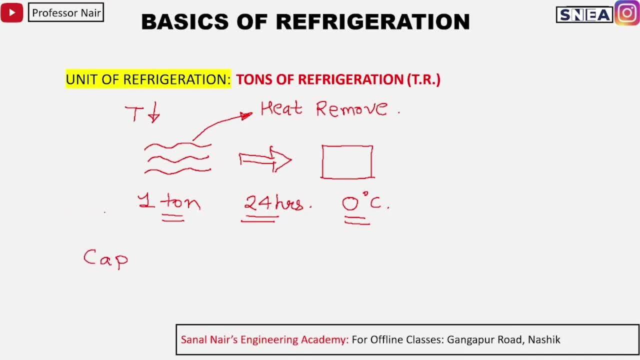 Okay, So are you understanding? So iska basic definition? kya hua, students? What is the basic meaning TR ka meaning kya? It is the capacity, Capacity to freeze One ton. Ek ton ko freeze karne mein kitna heat lagega. 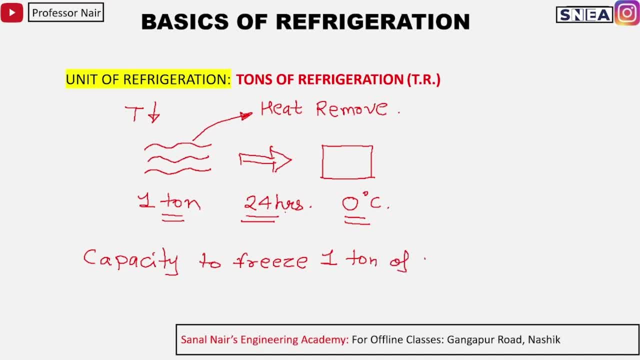 Kitna capacity lagega. That will be refrigerating effect. So capacity to freeze One ton of water from and at- This is an important wording- From and at How many degree Celsius? students, Zero degree Celsius. In how many hours? 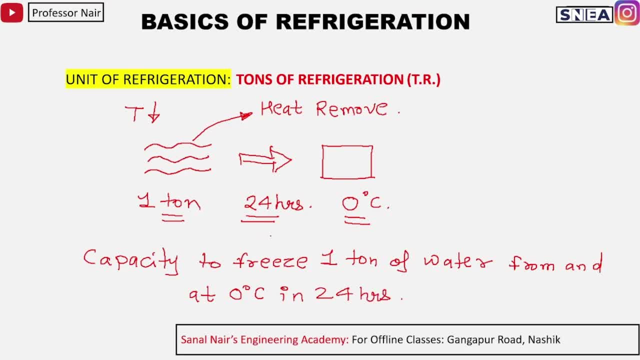 In 24 hours. In 24 hours. That will be termed as. that will be called as tons of refrigeration, That will be called as TR: One ton of refrigeration. So aap dhyan Do yaha par ki ek ton, agar aapko water ice mein convert karna hai. 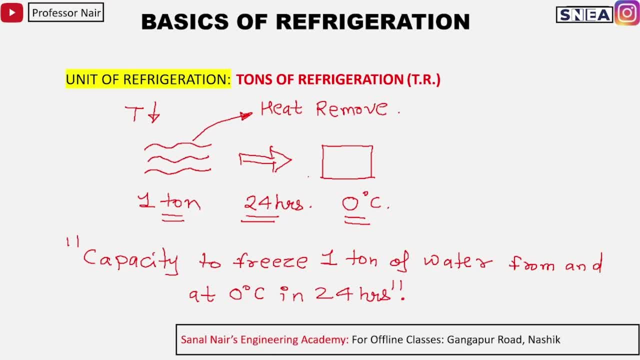 So it will require more amount of energy To bhai kitna amount of energy ke zurwat padti hai. So according to the law here, 1 TR yields 3.517 kilojoule per second. So iska actual meaning kya hai? 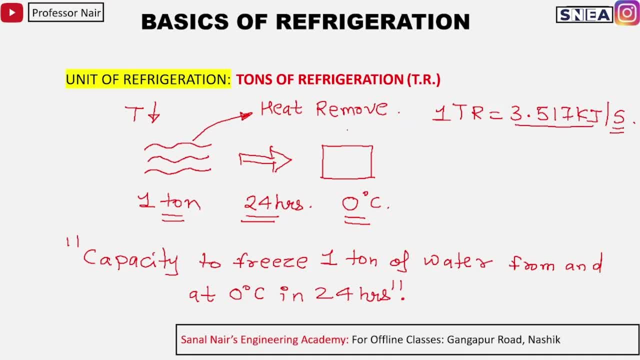 Ki ek second mein aapko kitna heat remove karna padega, students: 3.517.. 517 kilojoule heat remove karna padega. In how much 24 hours? Agar aap 24 hours mein 3.517 kilojoule remove kar rahe ho, ek second mein. 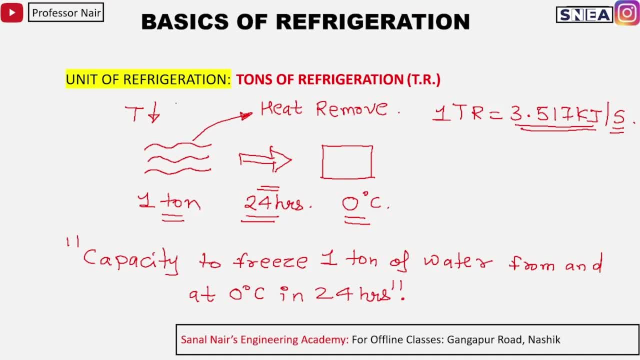 So us capacity ko kya bolte hai. Us capacity ko hum tons of refrigeration bolte hai. That is called as 1 TR. 1 TR equals to 3.517 kilojoule per second. Ek kilojoule per second matlab kilowatt. 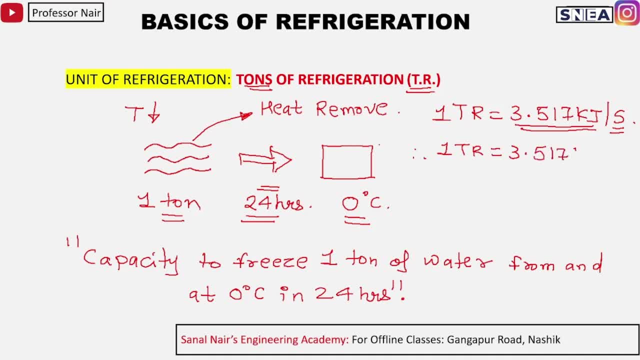 So it can be also termed as 3.517 watt students kilowatt. So yeh to second mein hua. Sometimes TR is also denoted in minutes. Minutes mein bhi hum isko denote karte hai. So generally it is of 211 kilojoule per minute. 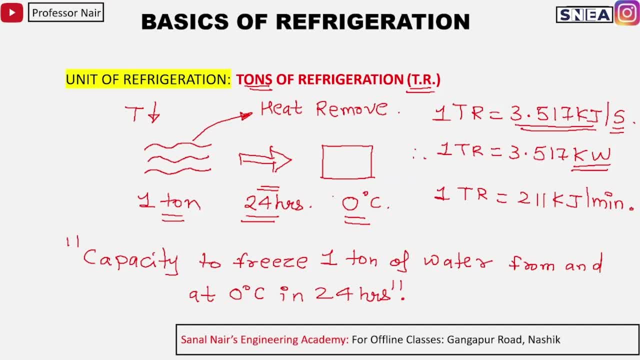 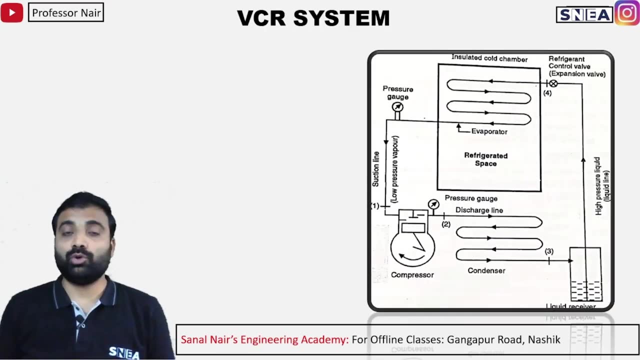 In terms of minute students, it is 1 TR, 1 TR matlab, 211 kilojoule per minute. I hope that you are understanding the basic of it very properly. At the start of the lecture, I have told you that we are going to study about what refrigerator 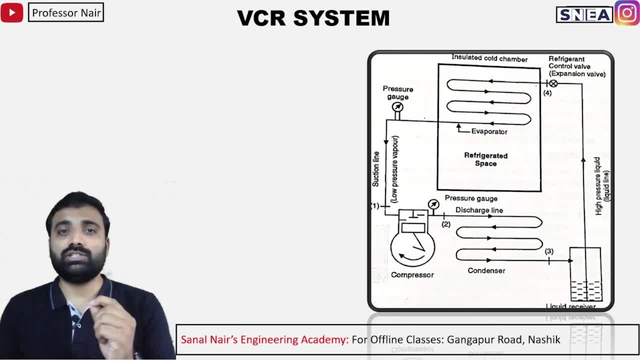 Ki refrigerator. mein system kya rehta hai? Refrigerator: kaise chalta hai How the refrigerating effect occurs? So, instead of cooling, we are going to use a very proper wording: that will be refrigeration. So, as you can see here, this is a system. 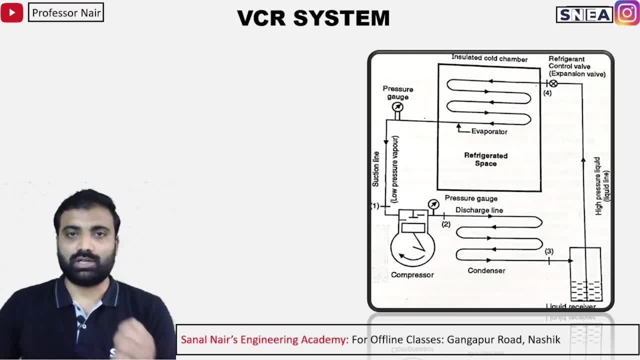 Okay, this is a system where a refrigerator works. So in this system sabse pehle to hum. dekhte hai ki kitta device hai. So first you can see, here we have compressor, Secondly, we have the condenser part. 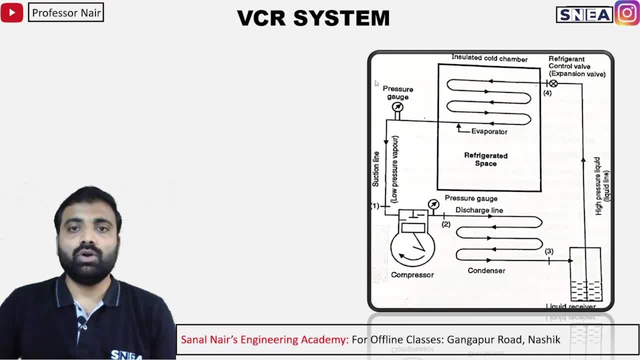 Second condenser, hai. Third liquid receiver. Fourth, we have the expansion wall, Aur jo. fifth device, hai students, that is evaporator. So we will go here step by step. We will understand the important point. It's related to this. 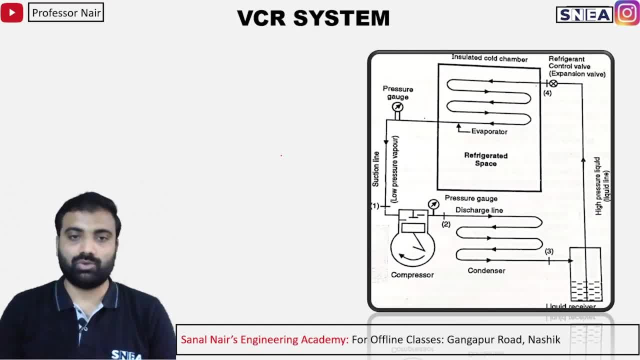 Samajh lete hai ki refrigeration ka process kaise occur hota hai. So the first device here is what students? It is compressor. Compressor ka main function kya reyega? Compressor ka main function reyega to compress the vapor. 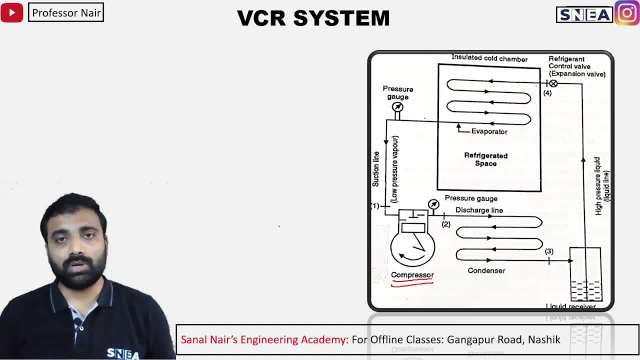 Vapor ko wo compress karenga? low temperature, low pressure se high temperature, high pressure me. So as you can see here the point one, Point one: me jo pressure aane wala hai. That is what Low pressure vapor Jo vapor evaporator se aega, that vapor will be what students? 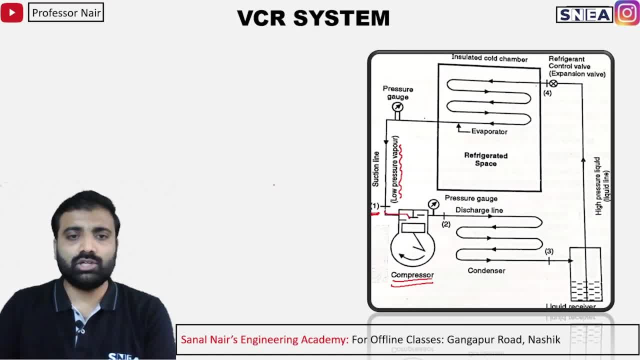 That vapor will be of low pressure. So when it enters into the compressor, when it enters into the compressor, compressor, us vapor ko compress karega. He is going to compress that vapor, students, due to which, at point two, at point two, jo temperature, reyega, aur jo pressure, reyega, that will increase. 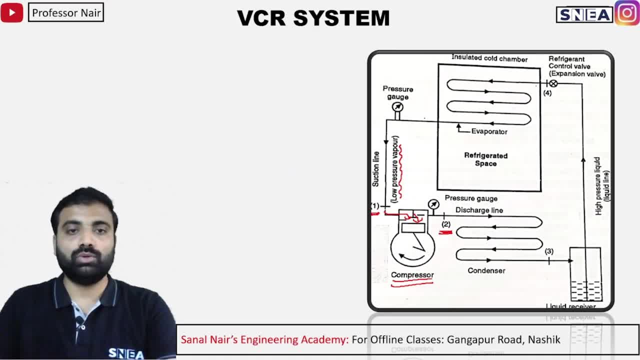 So what is going to happen in point one to two? What is going to happen in point one to two, One to two, me generally process, compression, karega. So one to two. I will write here which process it is: students: Reversible adiabatic process. 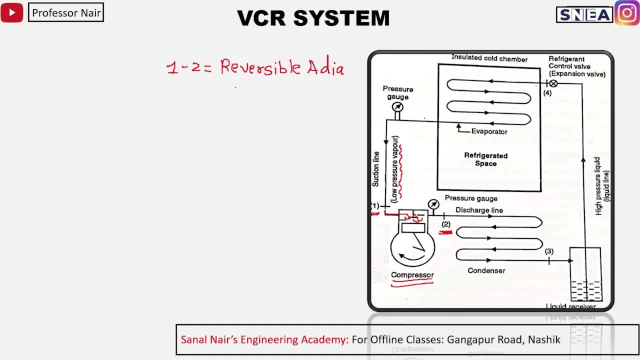 Okay, perfect, So reversible adiabatic compression ka process hoga. Adiabatic is ka meaning? kya hai? When there is no removal of heat, Heat, agar bahar nahi jayega. When Q dot is zero, then that will be called as what students. 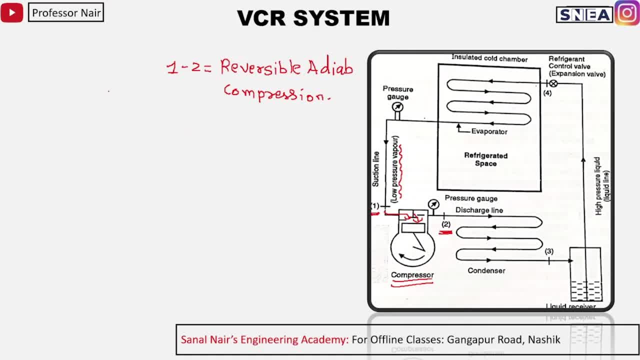 Adiabatic process or one to two compression. Okay, So in this case, what happens? in this case, Your low temperature, yaha pe dhyan do Low temperature vapor, Kis me convert, hone wala students, It is going to convert into high temperature, high pressure. 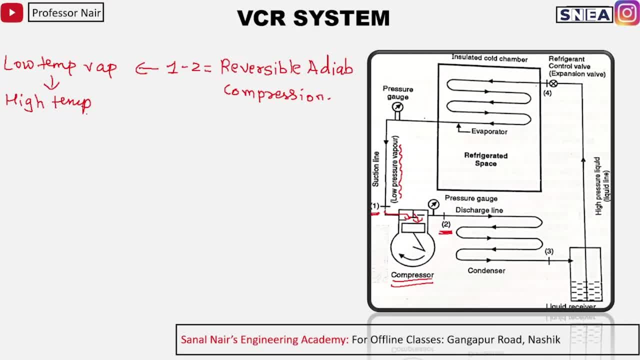 Okay, High temperature or high pressure me, kya hoga? High temperature, high pressure me convert hoga. That is your process, one to two. Okay, So that high pressure, High temperature, vapor will flow, will flow in the condenser. 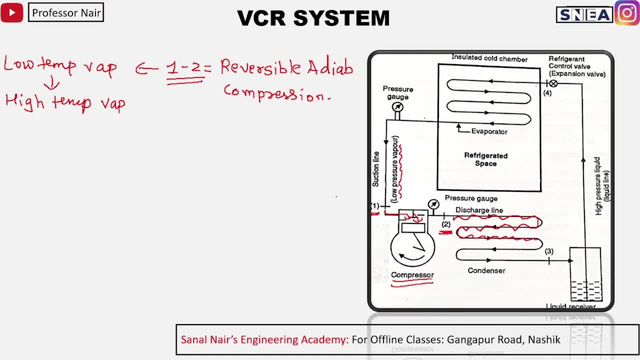 Okay, So condenser. as you can see, refrigerator me kaha per locate hota hai condenser. It is located at the backside of the compressor. Compressor ke backside me condenser rehta hai. So in condenser ye jo high temperature, high pressure hai, the vapor will give its temperature outside. 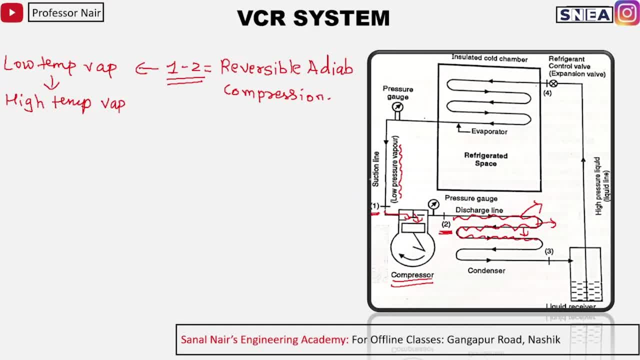 The vapor will give its temperature. Uske wajah se kya hoga? Vapor ka jo conversion hai, wo liquid me hoga. Means at point three, which state we are going to obtain Liquid state. Vapor se liquid state me kese kya hone wala hai. 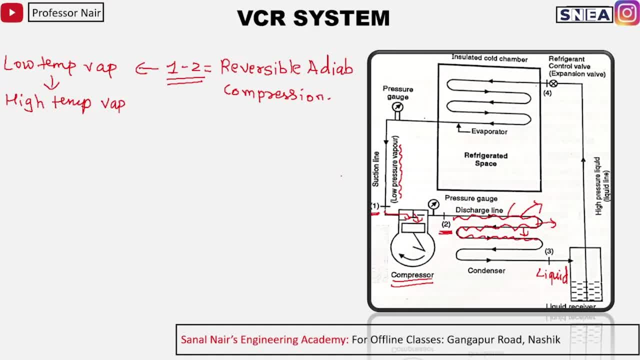 It is going to occur because of rejection of what students? Rejection of heat. When you are rejecting heat, you are lowering the temperature. Agar vapor ka temperature lower hua, it will get converted into liquid. So the Main function of condenser is to what student is to convert the vapor. 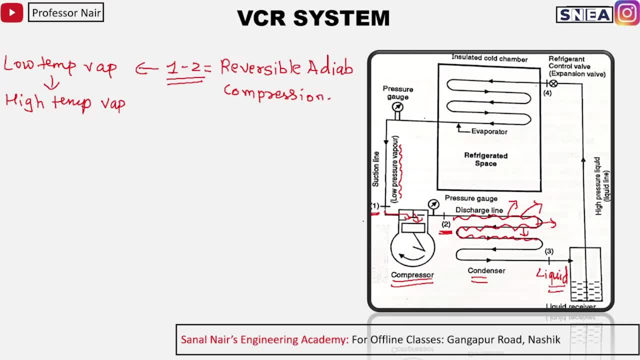 Vapor ka conversion kis me karega, Liquid me karega. Vapor ka conversion, liquid me karne wala hai. So, as you can see, the process 2, 2, 3.. As you can see, process 2,, 2, 3 will be called as what students will be called as the condensation process. 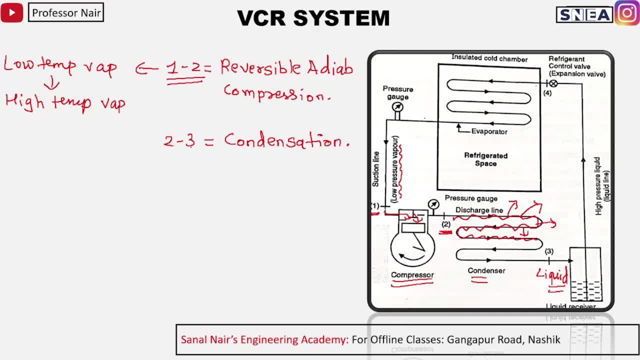 It will be termed as condensation process. So in condensation process liquid get converted into Sorry, vapor gets converted into liquid. Vapor ka conversion liquid me hone wala hai. Okay, But being the diameter same, point 2 se lekar. point 3, matlab expansion water. 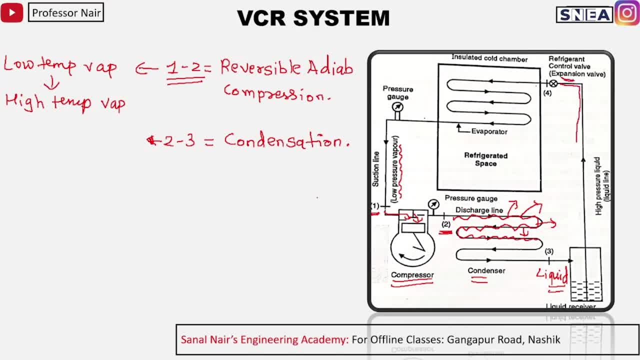 Aapka jo diameter, hai students. That diameter is going to what? That diameter is going to remain constant. That diameter is going to remain constant, So, due to which the pressure will be also same. So 2,, 2,, 3 me, there will be what. 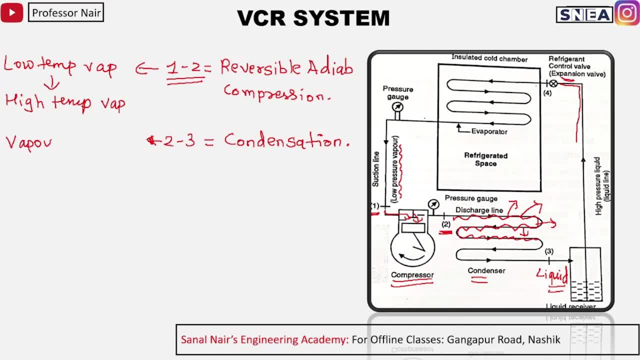 There will be conversion of vapor to liquid Perfect. Chalo, yeh toh samajh gaya. Liquid receiver me kya hoga? Liquid receiver me liquid store hoga, Okay, And that high pressure liquid goes into expansion wall. 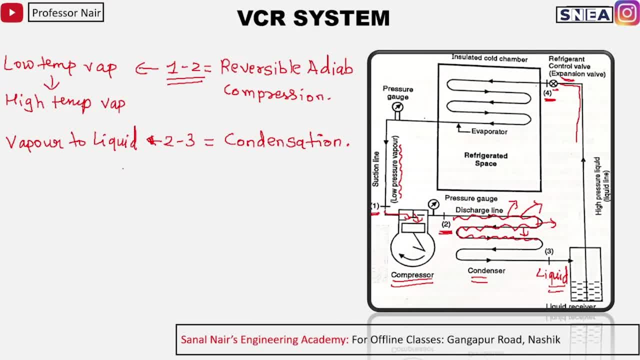 Fourth point: kya hai students Expansion wall? So let us see now what happens in 3, 2, 4 process. 3, 2, 4 jo process- reyega. that will be called as what students Expansion process. 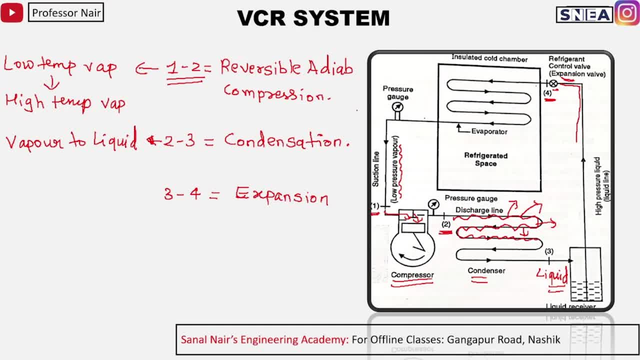 Okay, So at 3 point it is in which state Kaunse. state me hai students, wo It is: at high pressure, low temperature vapor. High pressure, low temperature vapor me hai students. Okay. So that will enter into expansion wall. Abhi generally dekho. 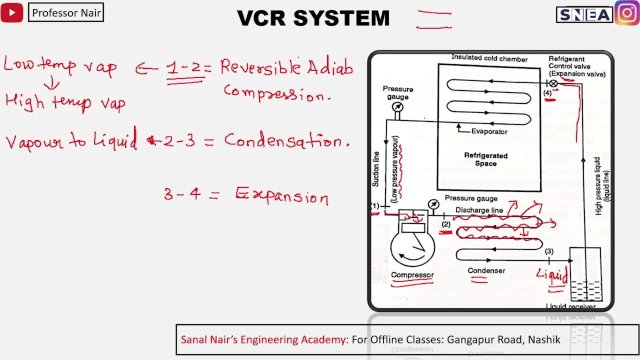 Yeh jo diameter hai. The diameter is like this. for example, If it is entering into expansion wall, Its diameter, what students? Its diameter reduces Matla diameter. kya ho raha hai Diameter? reduce ho raha hai Jiske wajah se pressure. 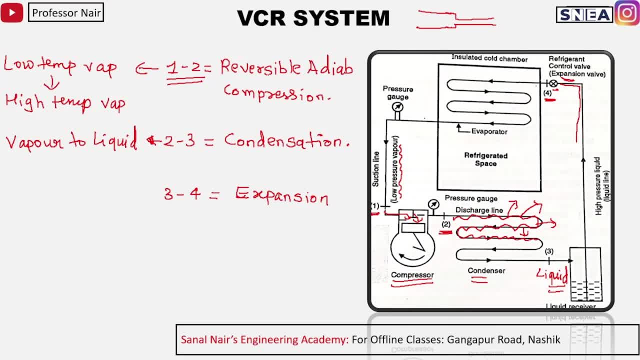 Uska decrease hoga. Bohot saare students ko yaha per confusion hota hai ki, sir, pressure kese kya decrease hoga. Pressure to increase hona chahiye As the area decreases. See the amount of liquid particle passing from here will be less. 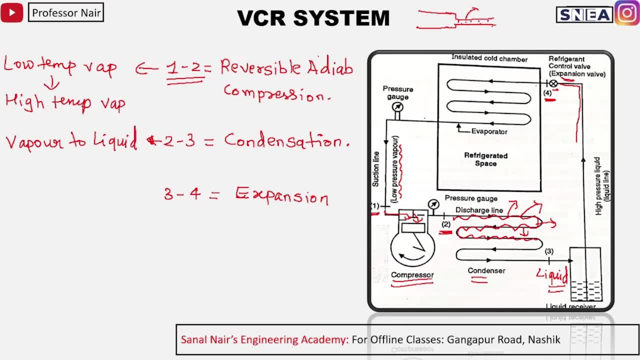 So it will exert a very less pressure Aur firse wo temperature bhi kya karega, Firse wo temperature bhi bahar emit karega. So that is why, fourth point, jo reyega, Fourth point, me pressure kya convert hoga? 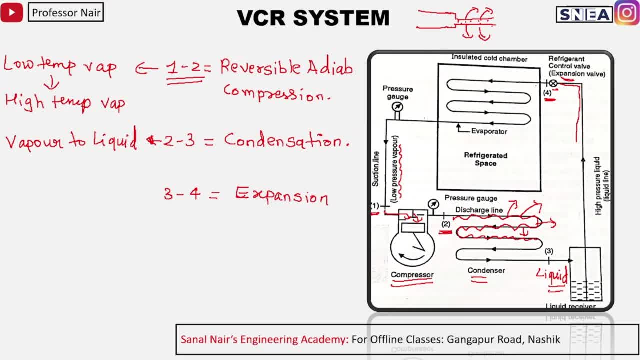 High pressure ka conversion, low pressure me convert hoga, while your temperature again reduces students Temperature. aur kya hone wala hai? Temperature reduce, hi hone wala hai. Okay. so in 3 to 4 there is your conversion process. Okay, which conversions happen? 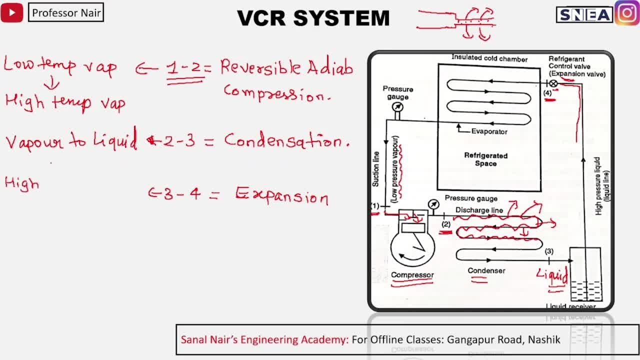 Which conversions happen: High temperature and pressure liquid. Okay, it will remain in liquid state only. It will get converted. Into what, students? It will get converted into low temperature and low pressure liquid itself. It will be in which state. It will be in liquid state. 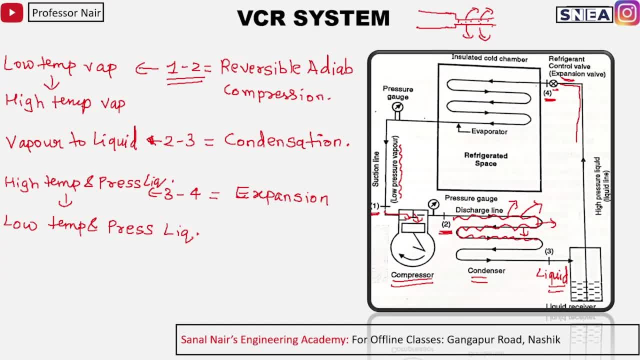 Woh liquid state me hi reyne wala hai. Dhyan do At fourth point: it will be in liquid state only. Perfect. But uska jo condition hai, Woh condition change hoga. High pressure, high temperature ka conversion, low temperature or low pressure me hoga. 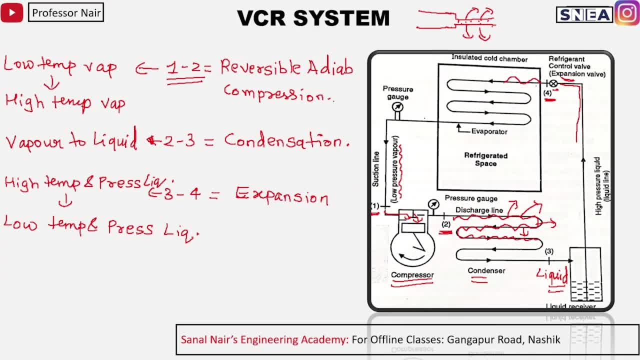 And then This liquid will enter into one of the important components of refrigerator, that is, evaporator. Phir ye jo liquid hai. ye liquid enter karega evaporator me. Okay, So, evaporator, kaha par situated hai? The evaporator is situated inside the refrigerator top compartment me. 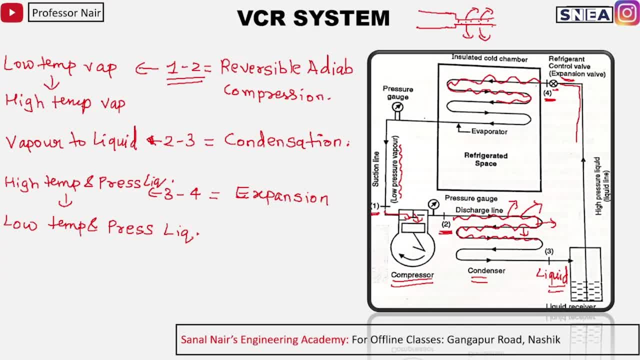 Jaha par ice cube form hota hai. If you will see that top portion, You will see a coil. Aap coil dekh sakte ho waha par, That coil Will be what students? That coil will be evaporator coil. 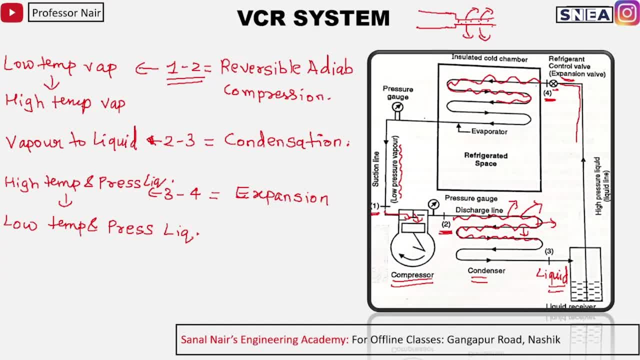 So us coil ko hum evaporator, coil bolte hai students. So what happens in evaporator? Let us see Theek hai Chalo Liquid to aara hai, But inside refrigerator we keep an object. Again, we will consider here the apple. 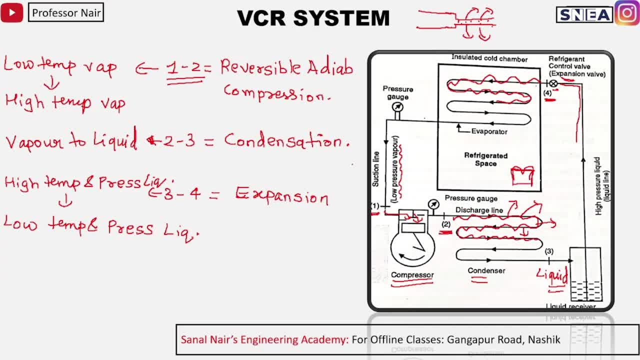 Okay, Apple, consider karte hai. Ya phir ek object, consider karte hai students. We will consider here the object. Okay, So the object is going to give the heat. The object is going to what students It is going to give the heat. 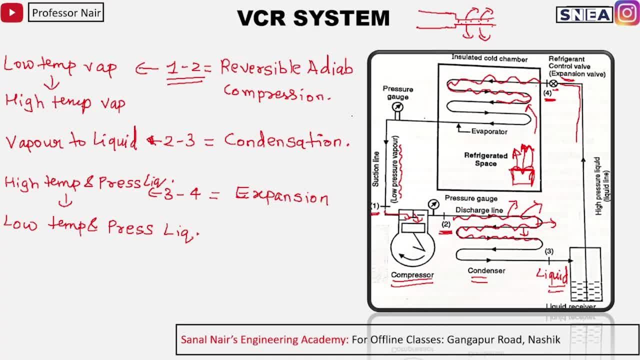 So ye jo heat hai. This heat will get received where? To the evaporator coil. Ye sab heat kaha par jaane wala hai. Ye sab heat jaane wala hai evaporator coil me. So when the liquid will receive heat? 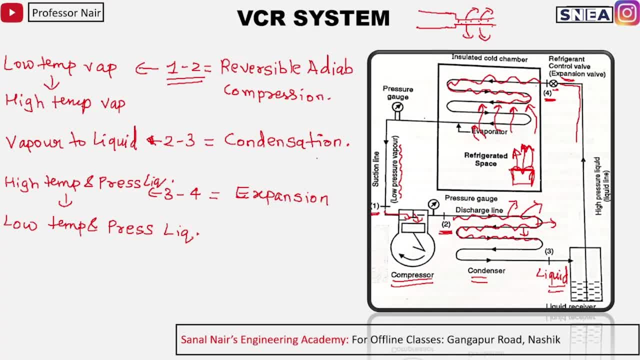 Agar kaunse bhi liquid me temperature, agar badega To liquid ka conversion, kis me hoga. Liquid ka conversion hoga Vapor me. So the liquid will get converted into vapor, Aur ye hi vapor kaha par jaega. 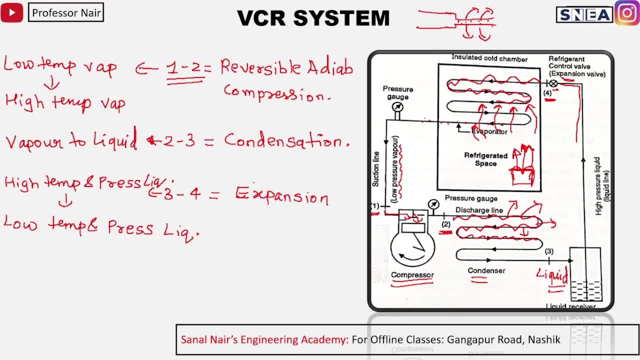 Compressor me and the cycle repeats: Dhyan do students? 4 to 1 is an important process. 4 to 1 is which process? It is a evaporation process. Which process students? It is evaporation process. Evaporation process me, kya hota hai. 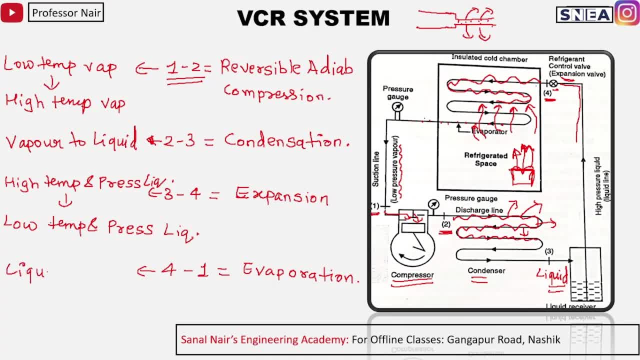 The liquid will get converted. Liquid will get converted to what Vapor? Phir se wo vapor me convert hoga. Abhi liquid ka conversion vapor me hone ke liye temperature ki zorwat padegi, So usse temperature kaha se receive hoga. 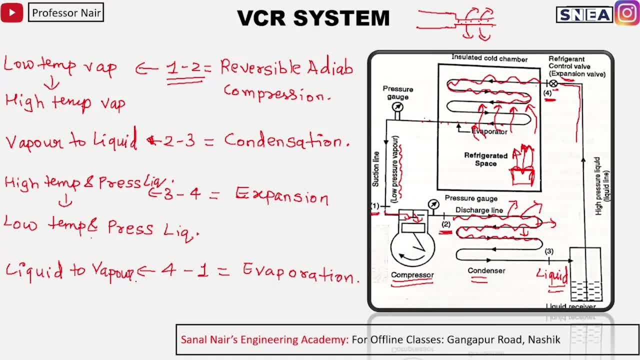 Usse temperature receive hoga ek refrigerated system se Ya fir ek body se jo refrigerator ke andar raka hua hai. So in short, again that liquid gets converted into vapor, Vapor compressor me jaake compress hoga, And the cycle. 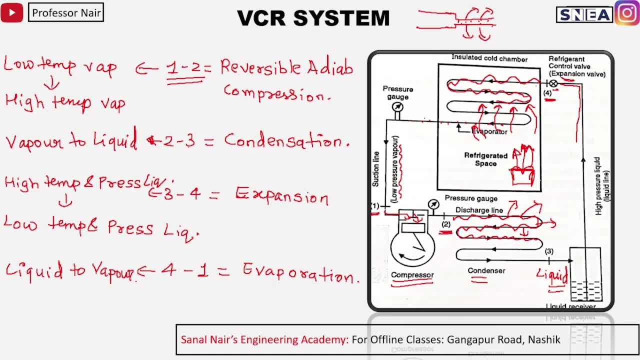 Keeps on repeating Means. if you will see here Ye jo do process. se condenser or evaporator Means condensation or evaporation, me Kya hoga? In condenser, vapor gets converted into liquid, And in evaporation, liquid will get converted into vapor. 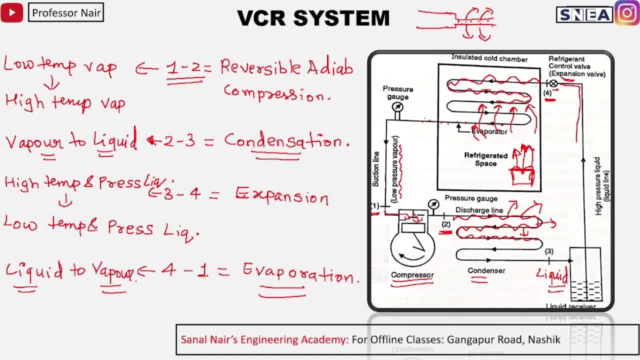 Liquid will get converted into vapor. I hope that you are understanding this process. Sabse pehle ye process samajh lo. Ok, I hope that you have pen and paper in your hand. Draw koro ye system. Ye sab point achche se likhlo. 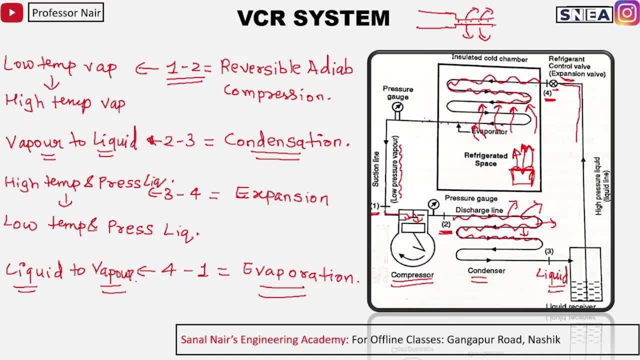 You can pause the video and you can write also here, So I hope that you are understanding. You have understood this system. that is VCR Vapor compression refrigeration system. This is your VCR system students, So we will revise what we had studied in VCR system students. 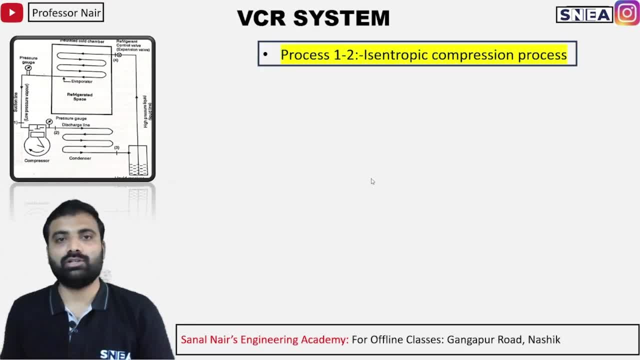 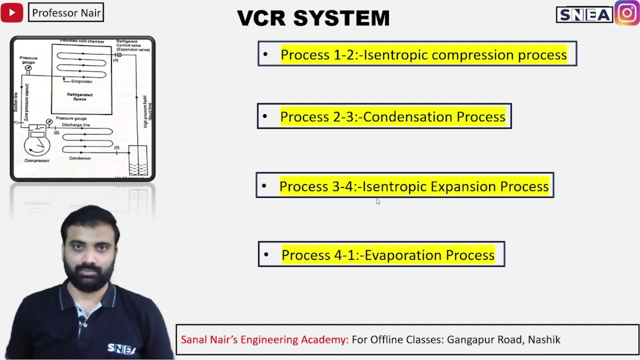 First process is your isentropic compression process. Process 2 to 3 hai condensation ka process. Process 3 to 4 is isentropic expansion process And process 4 to 1 is evaporation process. Ye total 4 process hai. 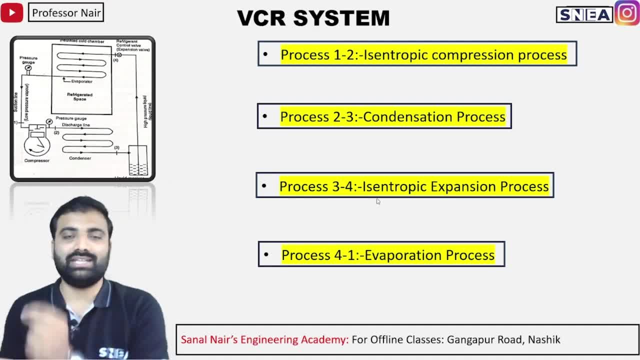 So all this process we have to plot on a pH chart. pH chart means pressure enthalpy chart. But before plotting this Whole process in the pH chart, Let us understand its meaning. Uska, actual meaning, kya reyega? Let us understand. 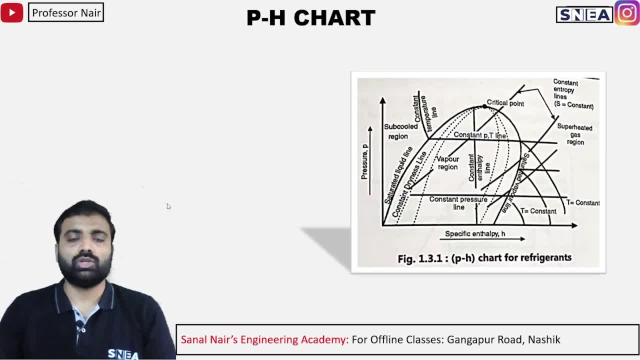 Let us go deep into that, Ok, So at this you are seeing here a pH chart, students, You are seeing here a pH chart. So this will be the basic. This on y axis will be. your pressure On x axis will be enthalpy. 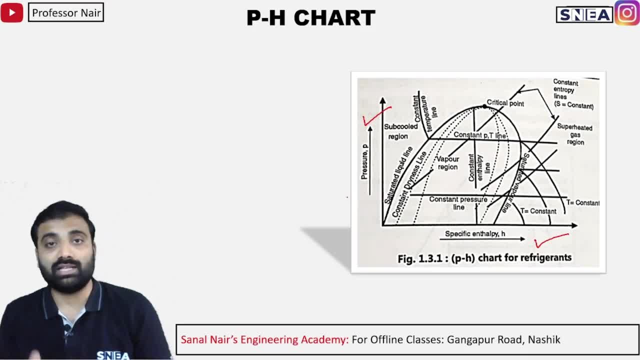 Specific enthalpy Means, in x axis there will be specific enthalpy, And on y axis there will be pressure property. If you will see here very properly, There is a curve here. Ye ha par a curve hai. So the curve on this side, here till the critical point. 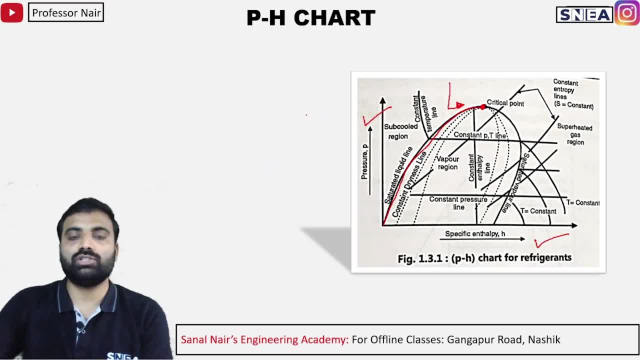 So this side of the curve will be your which region, students? That will be your liquid region, Means, if any point lies here on the curve, It will be of which region? It will be of liquid region, Ok, And if it is on this area. 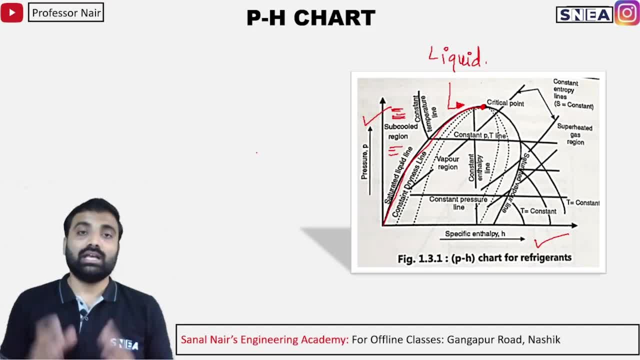 If it is on this area, That region will be called as sub cooled region. Sabse pehle to ye samajh lo That there is a liquid region And there will be a sub cooled region. students, Fine Aur right side mein aap agar dekho. 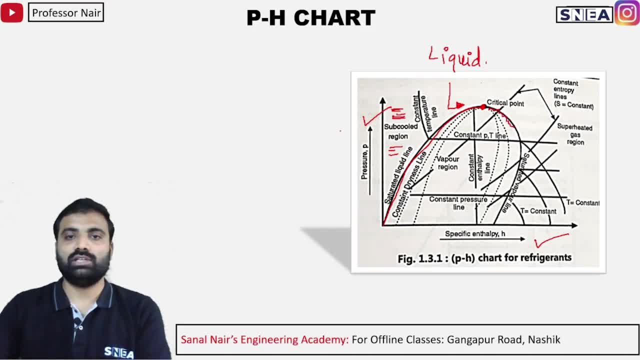 If you will see here on the right hand side, students On the right hand side here, If your point lies on the right hand side, curve That will be From which region. That will be your vapor region. So left side, mein liquid region. 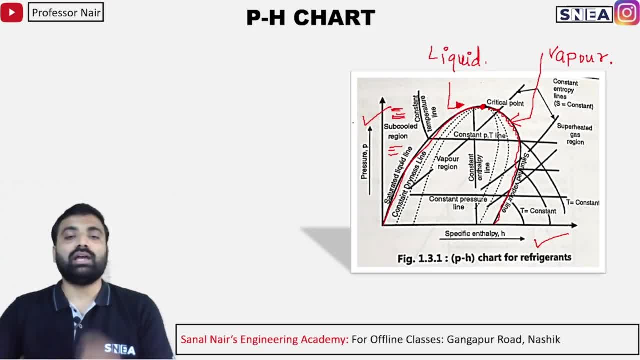 Right side, mein vapor region. So if my point lies on the liquid range, That will be liquid state. If my point lies on the right hand side of the curve, That will be on which state- Vapor state, rega Ek- liquid state. 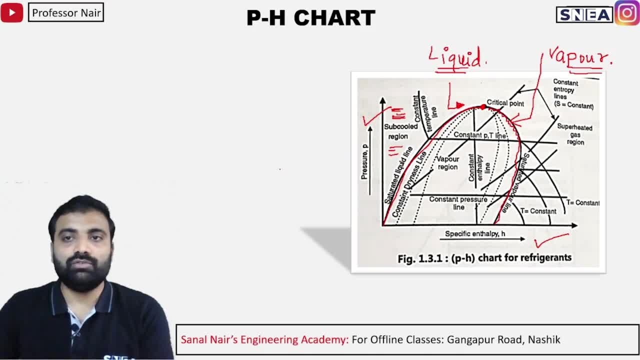 Ek vapor state rega, Ok, Perfect. So if my point, If my point lies here, Ok Lies here. Dekho dhyan do. If my point lies here, That will be your HF, HF. Iska meaning. kya hua students? 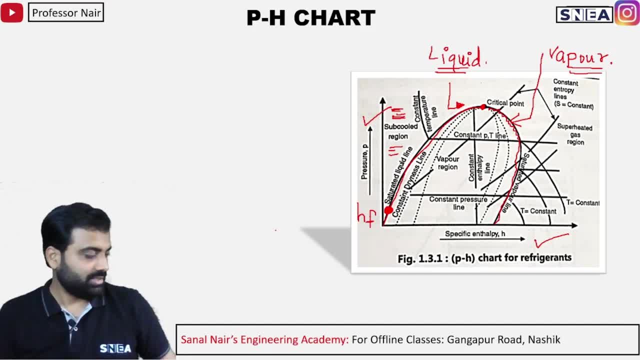 Enthalpy of fluid. In the similar manner, In the similar manner, If you will see here students, If you will see here That, if the point is where, If the point is here, Two minute students- Perfect. If the point is here. 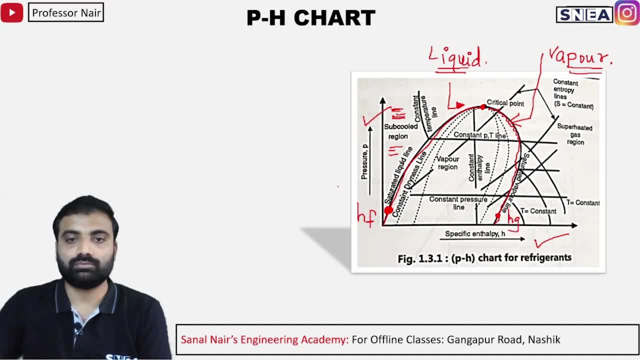 On this curve, It will be your HG. HG means what? Enthalpy of gas? Ok, HF, or HG- Enthalpy of fluid. I will just write down here: HF ka meaning ho gaya Enthalpy of fluid. 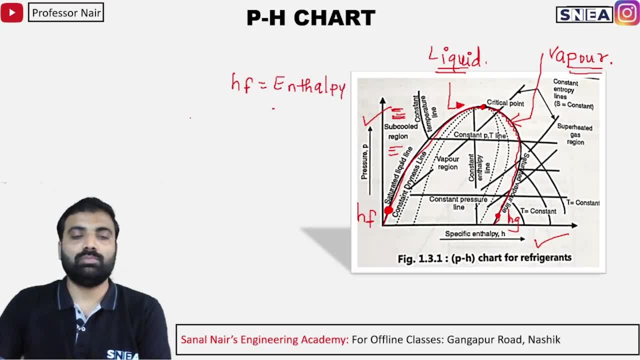 Fluid means your liquid Enthalpy, Enthalpy of fluid, students, or liquid Perfect, And here its meaning will be what It is, what HG. HG means what students. HG means enthalpy, Enthalpy of gas. 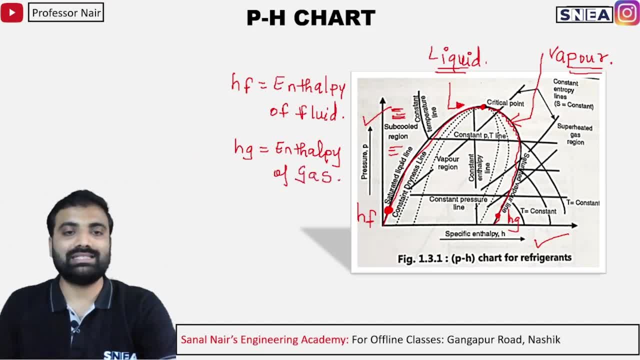 Enthalpy of gas. So, first and foremost, You should understand the meaning of what students HF as well as HFG. So let us see the next part. Ok, If here is HF, This is the HF part. This is the HG part. 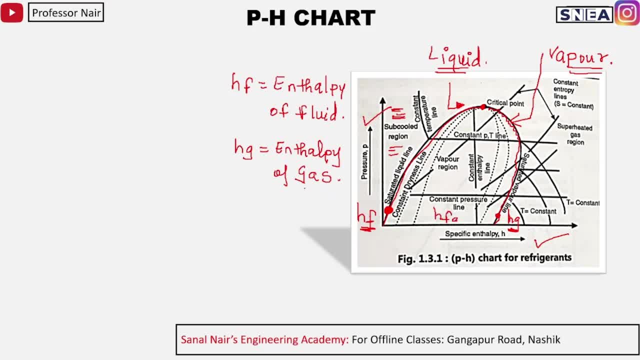 In between will be called as HFG. In between will be called as what students? HFG. Enthalpy of wet steam- That will be called as enthalpy of wet steam students. Enthalpy of wet steam students will be called as enthalpy of wet steam students. 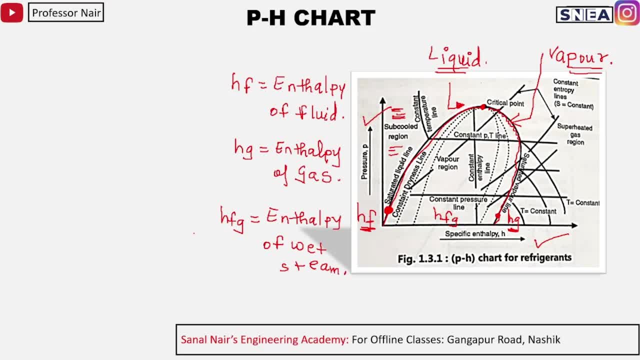 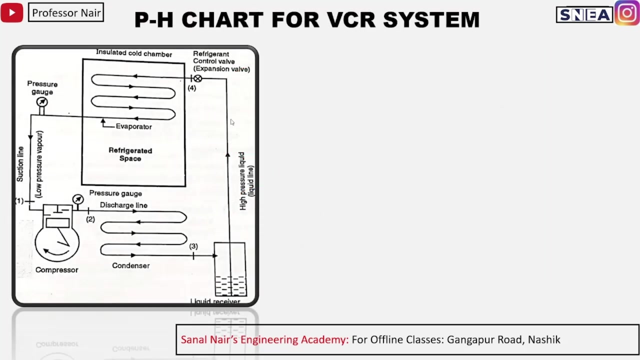 Are you understanding? So three important enthalpy I have plotted here: HF, HG and HFG. Perfect, Ok, So let us understand now that how I will plot the pH chart for this VCR system, How we will draw pH chart for VCR system. 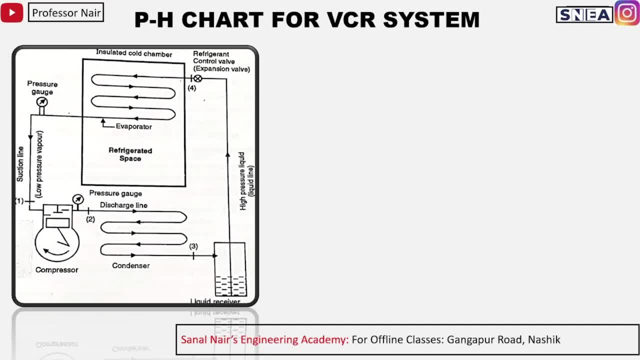 Ok, Ok, Ok, Ok, Ok, Ok. So first of all, I will draw here a y-axis. Secondly, we will draw here an x-axis. Ok, A y-axis or a x-axis. In y-axis, we will have pressure. 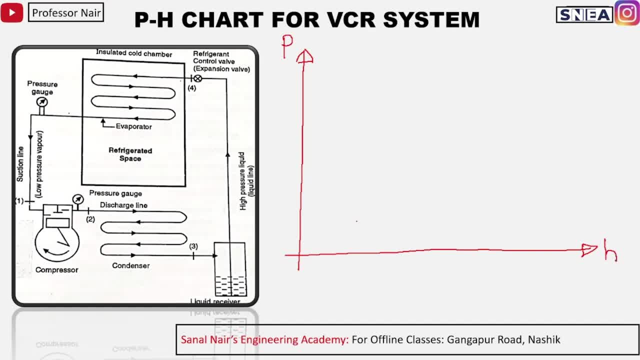 On x-axis, we will have students, enthalpy, A pressure, or enthalpy will be P, and what students? P and H. Ok, So let us draw the basic structure diagram. So the structure diagram I have just explained you now. 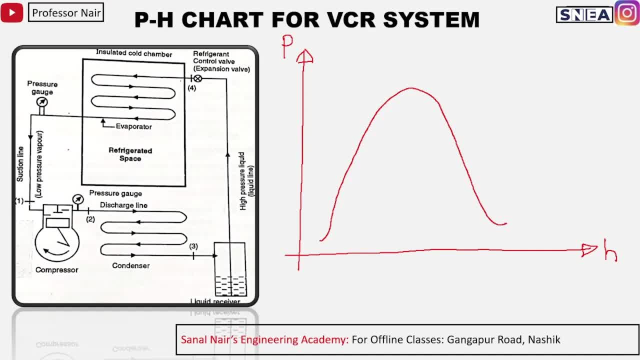 So this will be its structure diagram. Ok, So first point. Let us start with the first point. First point is in which state students are in vapor state. So the first point that will be in vapor state, that will be 0.1.. 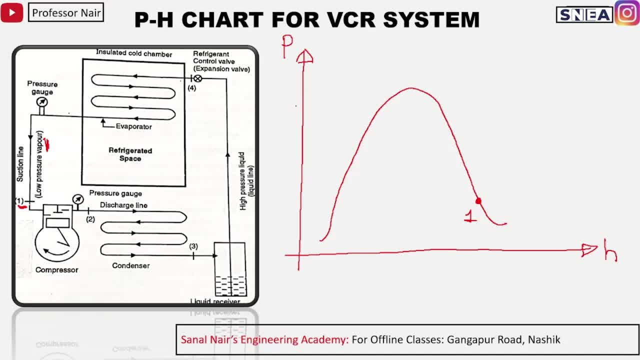 Are you getting this line? this curve will be for vapor. I will write it again: This curve will be for vapor and the left hand side here That you are seeing students, that will be your liquid. Ok, So one point: 1 to 2. what is happening? students? 1 to 2: compression is happening. 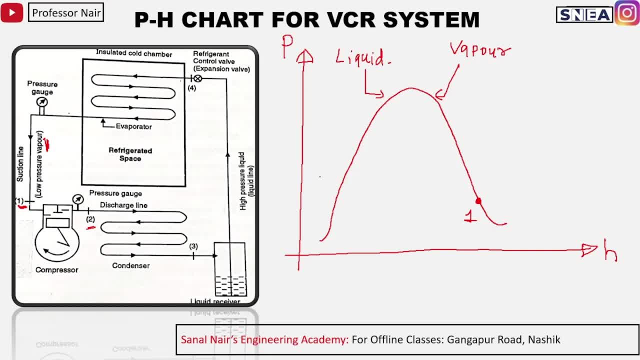 Compression is going to happen, So, due to which its pressure, as well as enthalpy, increases. So I will draw here like this. So this will be what, students, this will be point number 2.. Ok, So point number 2 is going on this region. 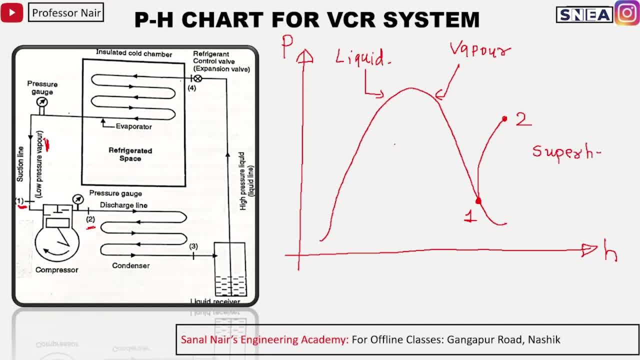 This region will be called as superheated This region. This region will be called as what students? superheated region will be Ok, great. So 2 to 3. what will happen? which process will happen? condensation: What will happen in condensation? 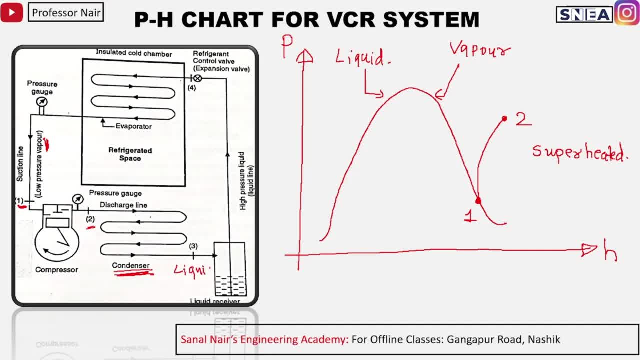 The conversion of vapor will happen in liquid. But I have told you. I have told you that in diameter, same means what will be the pressure. Pressure will be constant. So at constant pressure I have to show the vapor conversion into what? into the liquid. 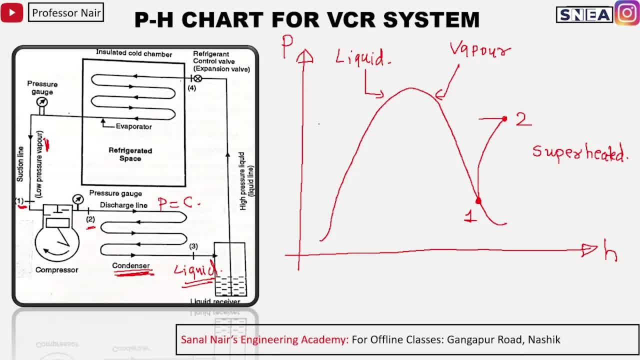 So the liquid is here. So what I will do? I will just draw a line here And the liquid will come. This will be which point, students? This will be point number 3.. So 1 to 2, this is your compression. 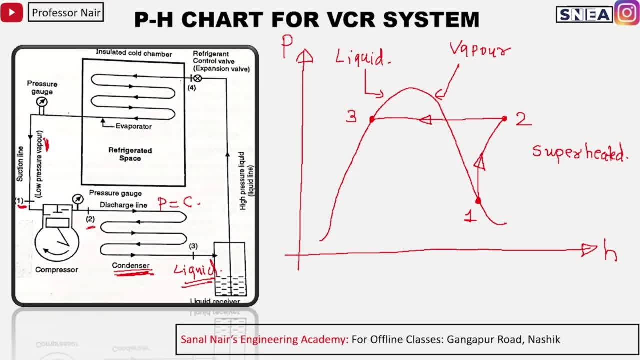 2 to 3. this is your condensation. So at 3 point it is in which state? liquid. Ok, So again here, the pressure will be constant as diameter is constant at point 4.. But what will happen? which process will happen? expansion. 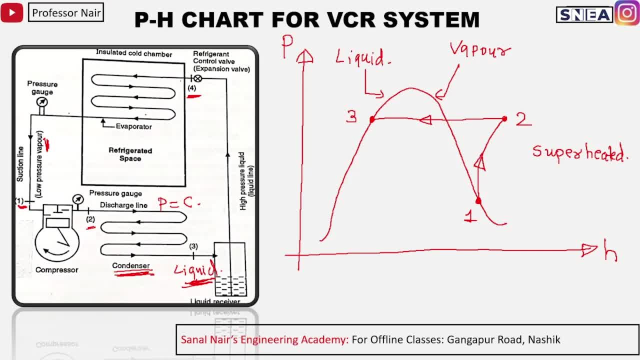 I have told you expansion process in pressure and temperature. both will be what will happen. Both will be less. Both pressure as well as temperature is going to reduce, it is going to decrease. So decrease in pressure, you will have to show, So this will be your which point? fourth point means the fourth point will be inside the liquid as well as. 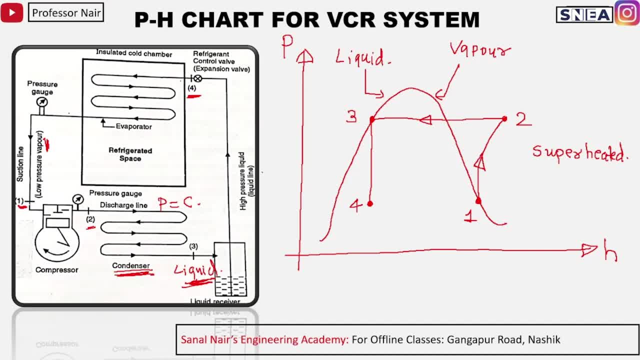 Vapor means which state will be that will be liquid, as well as what strands as well as vapor. Perfect, Now this point 4 will enter inside what strands? enter inside the evaporator. It will enter inside the evaporator, In evaporator. what is going to happen? 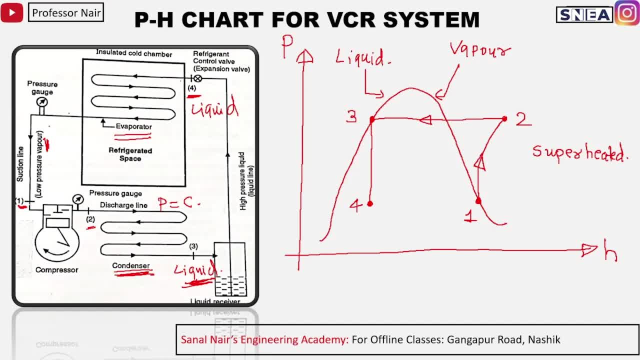 The liquid On which will be the liquid conversion. The liquid conversion will be in the vapor, As we have The refrigerated system inside That will give heat to the evaporator. Ok, So again from the fourth point, one point will have to come. 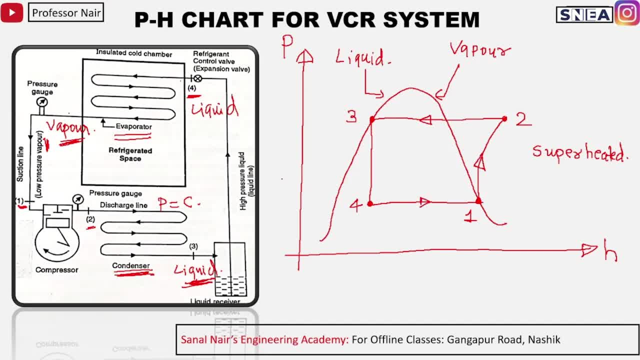 Pressure will be constant, So this will be again Evaporation process. So let us see 1 to 2. 1 to 2 is which process students, Compression. This is the compression. 3 to 2 is which process condensation. 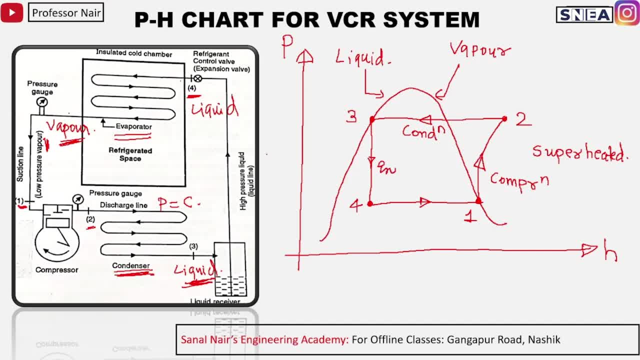 3 to 4 is which process. It is expansion. It is expansion process, And 4 to 1 is which process, It is evaporation. This will be evaporation. I hope that you are understanding it very properly. Point 1 to 2: compression. 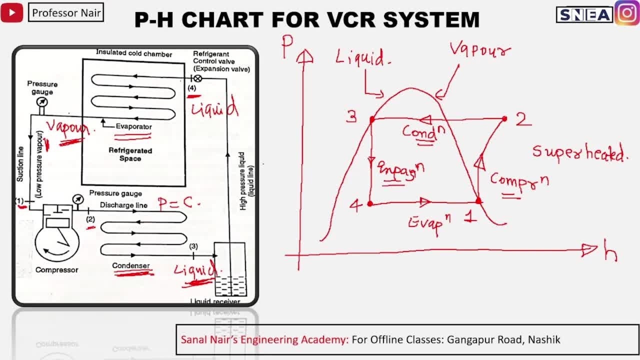 2 to 3 condensation, 3 to 4 expansion or 4 to 1 evaporation. But there are some different conditions, students. There are some different condition to achieve this. Ok, So this was all about VCR system. 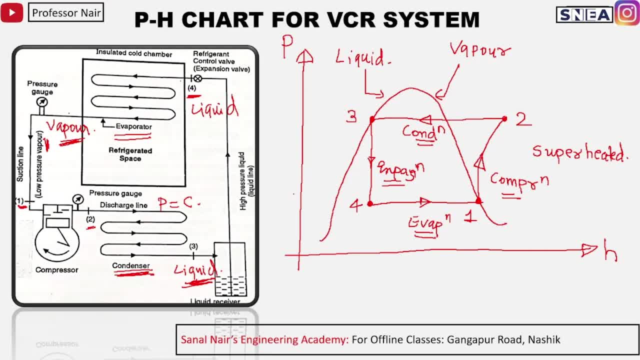 This we had studied about the VCR system. Vapor compression refrigeration. We have plotted the pH chart also. Now we will move on to the next part, next refrigeration system. That will be what students. that will be vapor absorption system. Vapor absorption system. 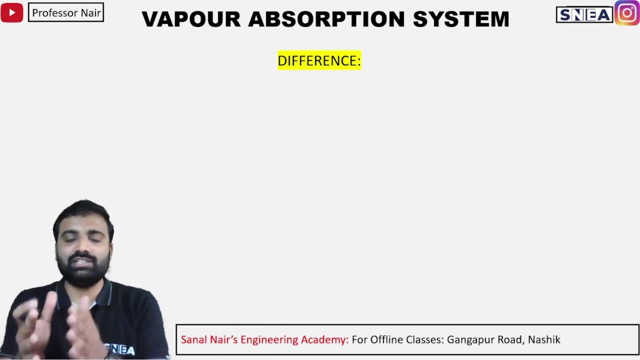 Ok, So the main, important, The important. The second thing here is: what students? What is the difference? What is the difference? What is the difference between vapor compression and vapor absorption? So the difference is in compressor, In vapor absorption system, you don't have compressor. 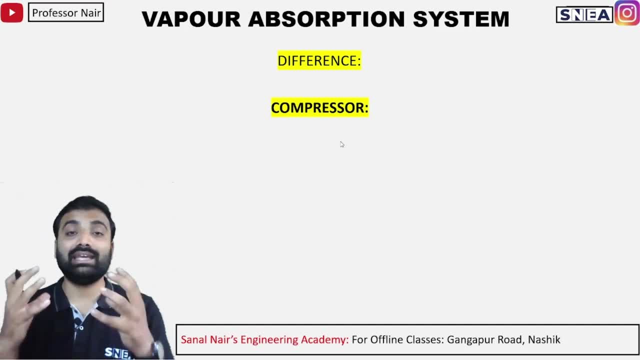 You don't have compressor, The compressor, that element is absent. So, instead of compressor, What we are going to use, What we are going to use? So, instead of compressor, We are going to replace it by 3 devices: Absorber. 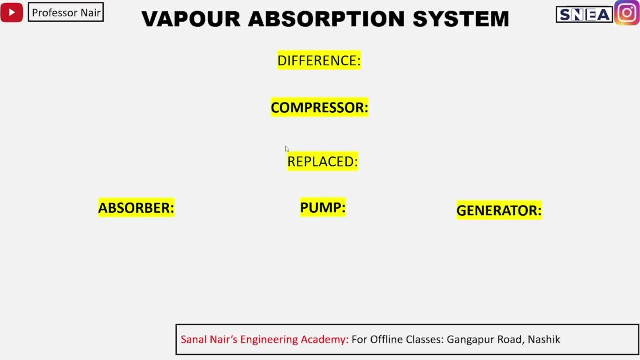 Pump And generator. These 3 devices, students, These are the 3 devices in vapor absorption that is going to replace. First of all, we have replaced the compressor with the absorber And the third one is the generator. Third one is what students? 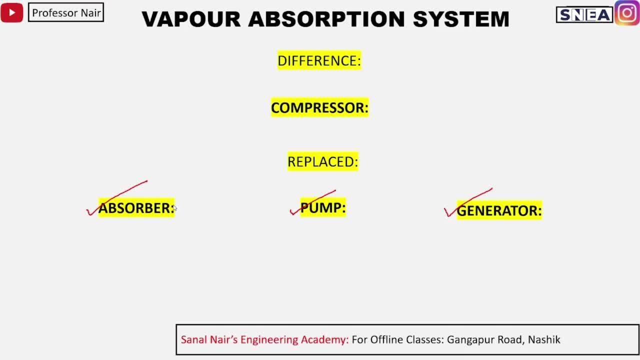 Third one is the generator part. Ok, So what does an absorber do? What does an absorber do? It converts the weak solution to the strong solution. Ok, Ok, Pump, obviously. what will it do? Pump will raise the pressure. 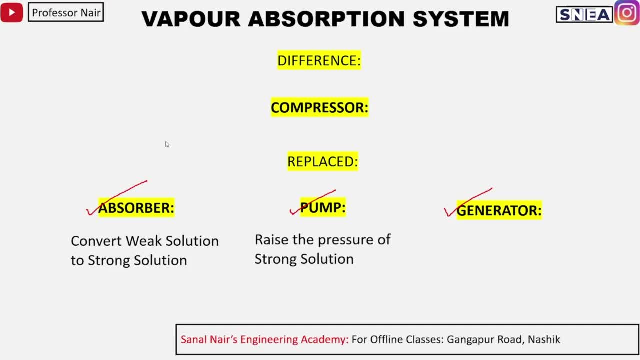 So it raises the pressure of strong solution. It raises the pressure of strong solution And generator, It converts the strong aqua solution. The compressor will now switch from a aqua solution to vapor: The conversion of aqua solution. What will it do, students? 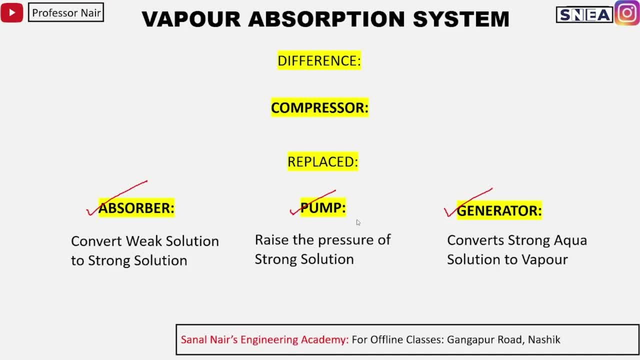 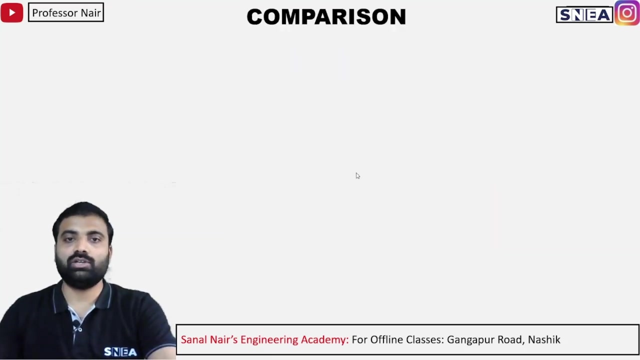 It will convert it into the vapor part. Ok, So VCR and VAS will have the most important difference: That the compressor that was used in VCR Will get replaced by absorber, Will get replaced by pump. This will be replaced by three devices and at last, just we will see the comparison between. 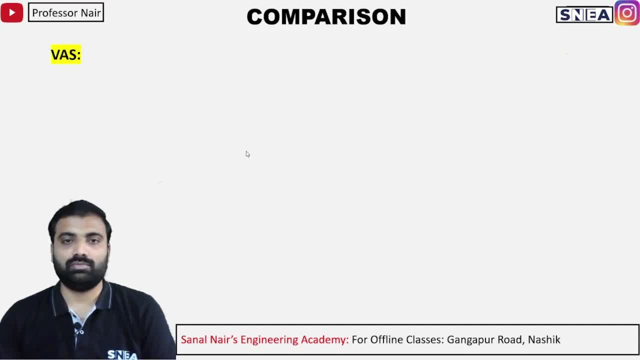 the two, VAS and VCR. So in vapor absorption system it uses low grade of energy, but in VCR, the energy we are going to use that will be of high grade energy. In vapor absorption system we have only one moving part. that is what students pump here. 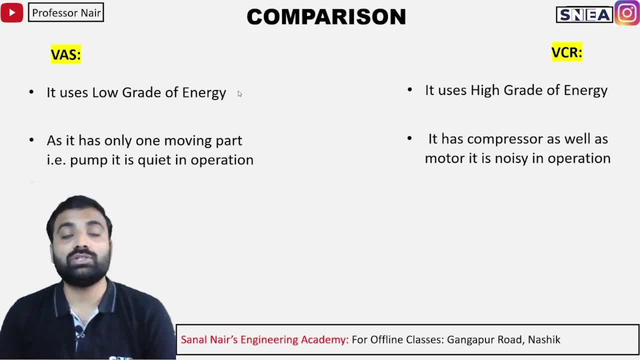 we have a compressor means in vapor absorption system. compressor is replaced by absorber pump and generator. So out of absorber pump and generator pump is only the noisy in operation, while here in VCR there is compressor. In VAS the possibility of leakage is less. 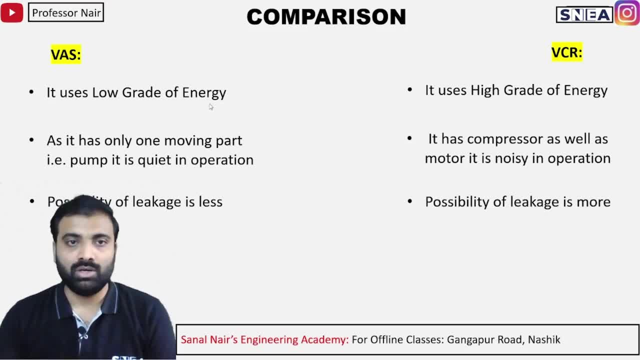 While in VCR the possibility of leakage is high and obvious, as we are using low grade energy. the COP, that is, coefficient of performance, that will be less as compared to what, as compared to the VCR system. So these are the basic difference between what, between the VCR and VAS students. 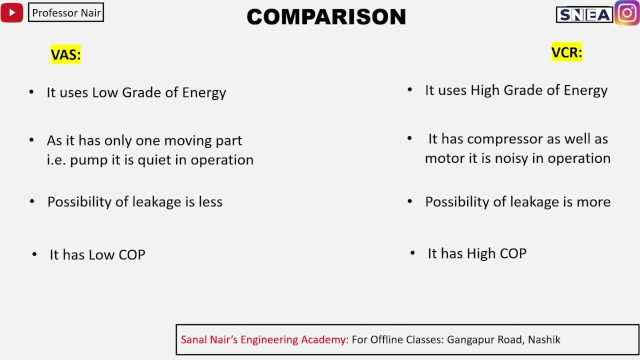 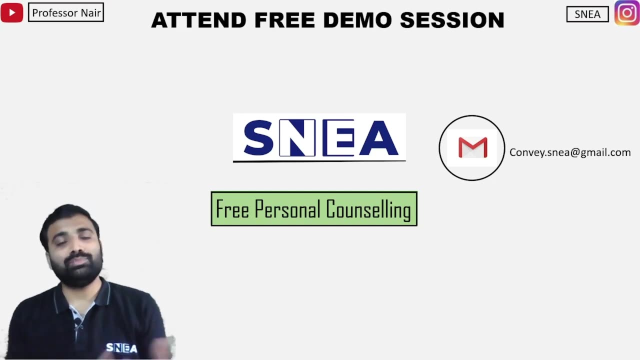 Leakage possibility will be less in VAS and leakage possibility will be more. It will have low COP. it will have higher COP, students. ok, are you understanding? So in this way we have completed the first part of the video. I hope that you have understood and if you have any doubt you can free to call me- that the number is been given in the. 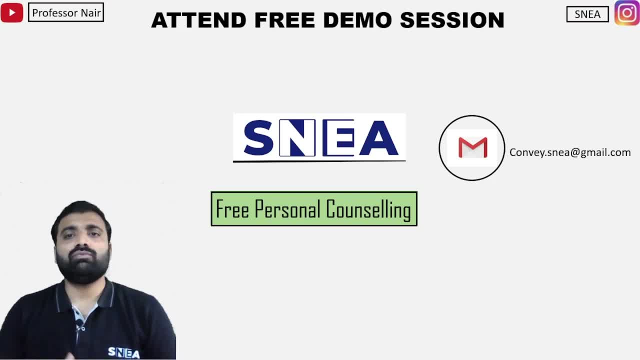 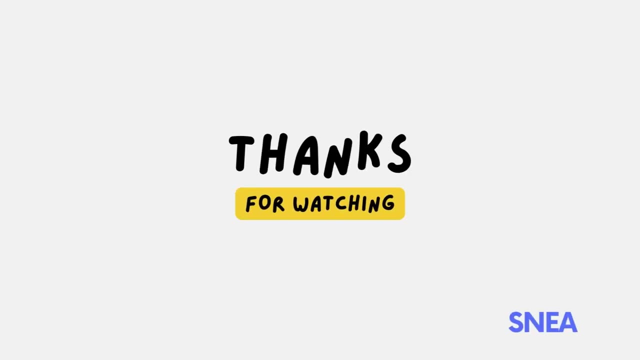 description. You can join the whatsapp group as well. In whatsapp group I keep on updating about the lectures, So it was a nice teaching. thank you so much, students.